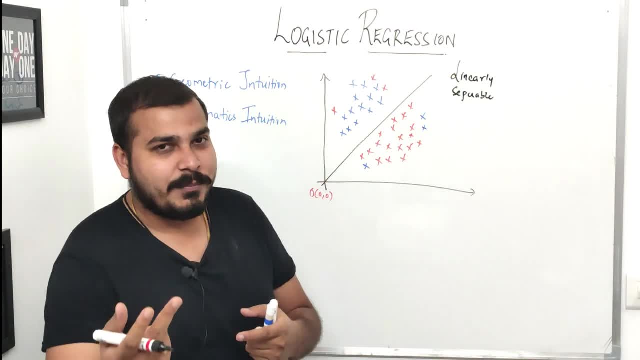 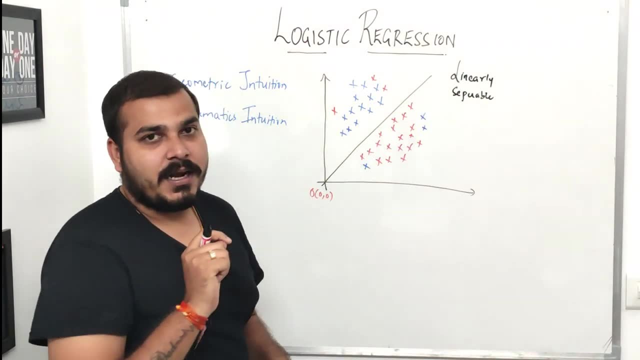 So this is basically a plane. If I just consider something like a two-dimensional graph at that particular point of time, I can call this as a plane. okay, So we need to actually find out this particular best-fit line, such that it will be able to linearly separate these two particular points. 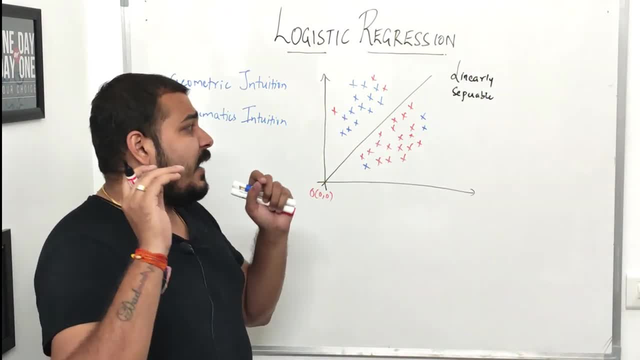 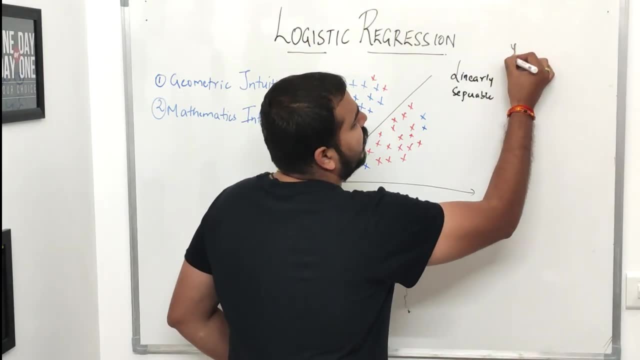 the classification points. Now, this is pretty much simple, guys, And you obviously know that whenever we are creating this particular straight line, the equation is pretty much simple. The equation I can write it as: y is equal to mx plus c, right? 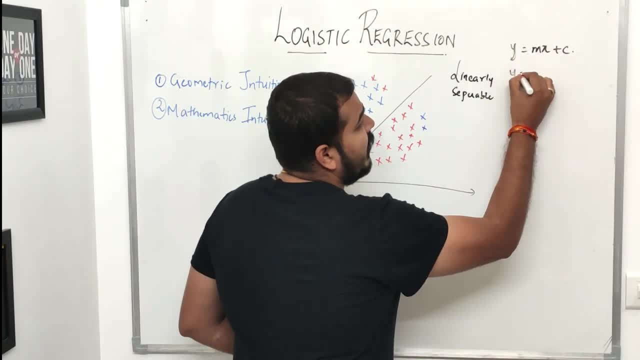 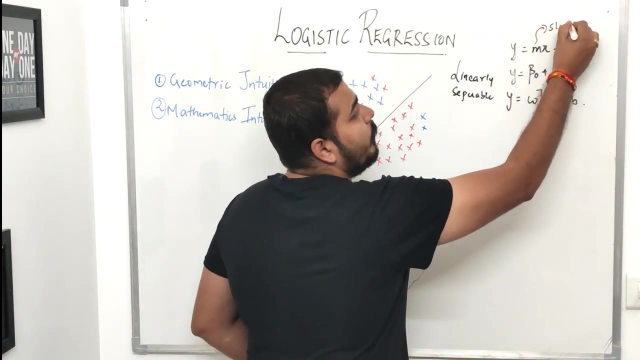 And there are some other notations also which I have already discussed yesterday. I can also write: y is equal to beta 0 plus beta 1 into x. y is equal to w, t, x plus b, right, Right, and I hope you all remember that this m is actually the slope. 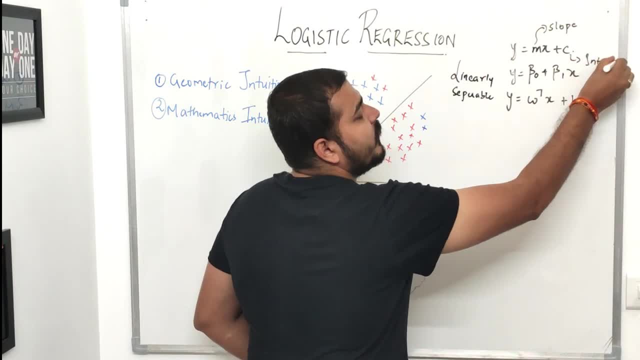 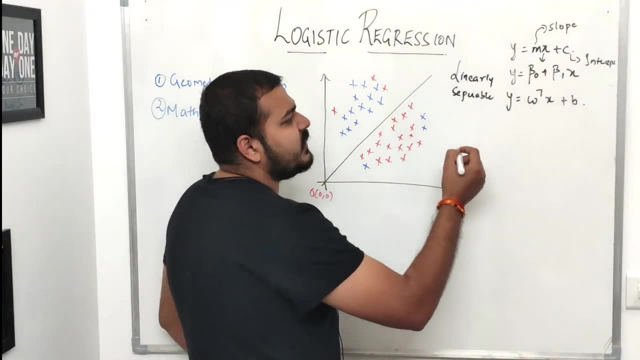 This is basically my intercept right And this x is my data points. okay, These are all data points, Right? I hope you have understood this. Now let me consider some equation. I can consider this. I can consider this also right. 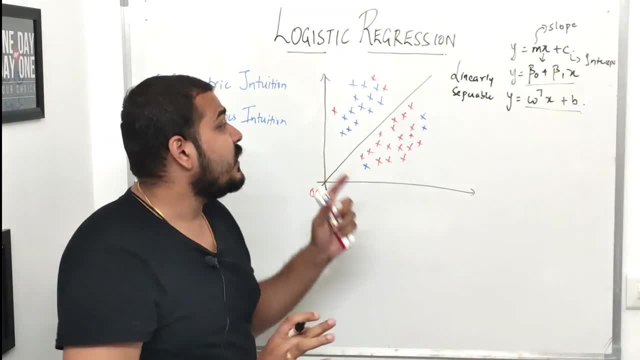 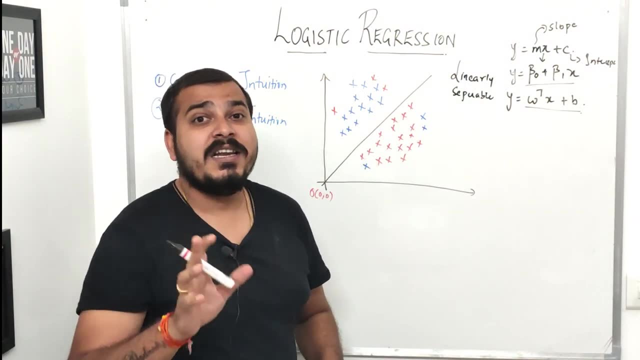 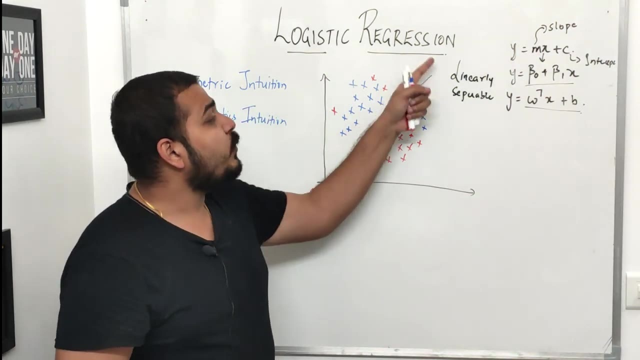 Now, always remember that. what is the important thing that you need to understand, because this does not work like linear regression. okay, The best-fit line is not calculated with the help of linear regression. There is some other way. We need to find out this exact coefficient which will be able to understand. 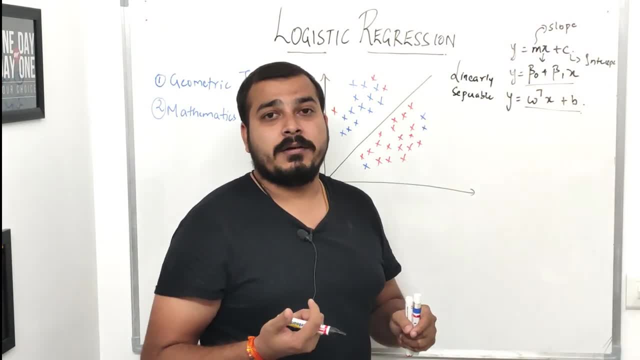 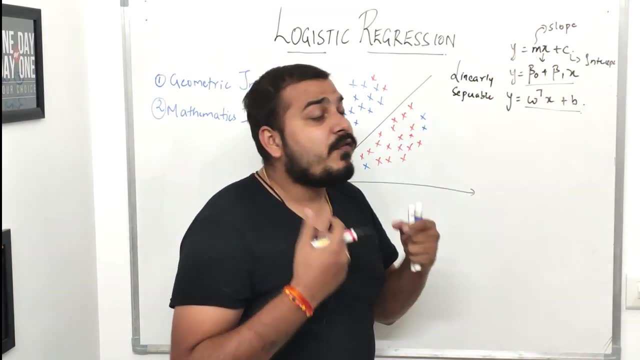 which is the best-fit line, and we need to modify this particular coefficient. okay, Coefficient dot slope: In this particular case, it is w. In this particular case, it is m. right, We need to find out this particular value, okay. 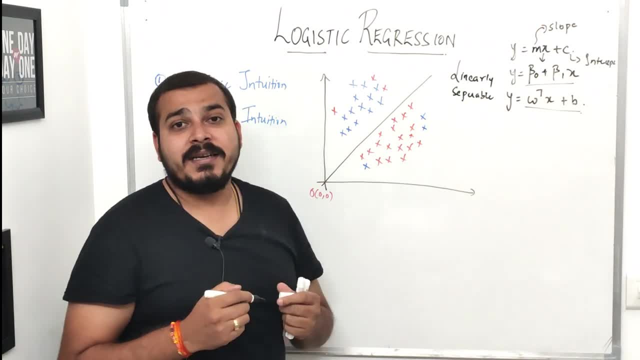 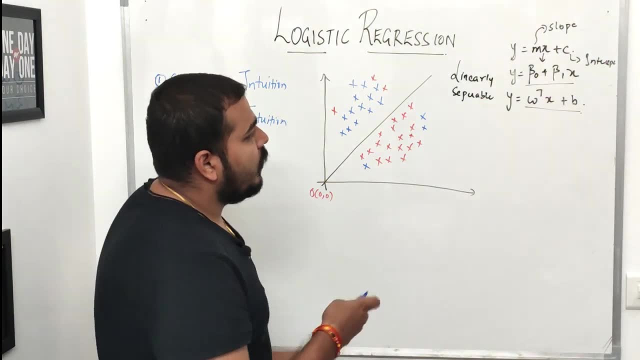 Now for doing that. how does it actually happen in logistic regression that we need to understand? okay, Now let me consider some of the assumptions that we usually do. is that for the positive points, that is, for this blue points, I am going to take it as plus 1, okay. 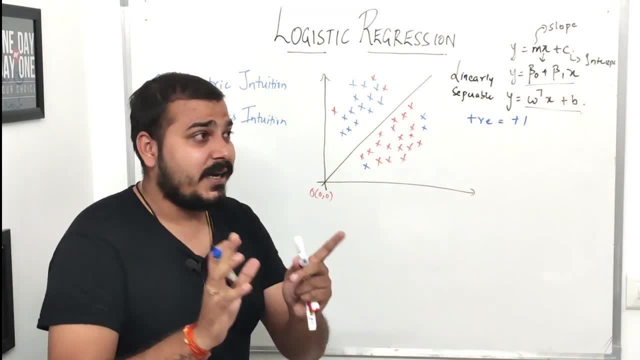 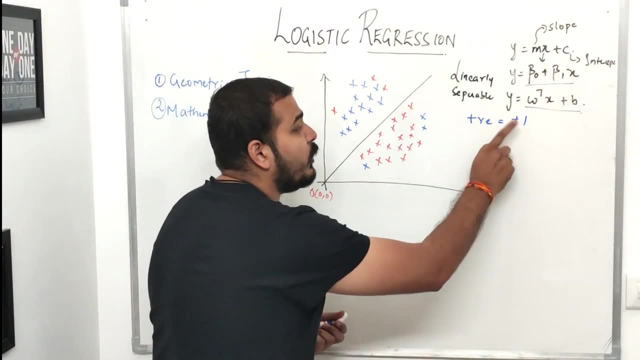 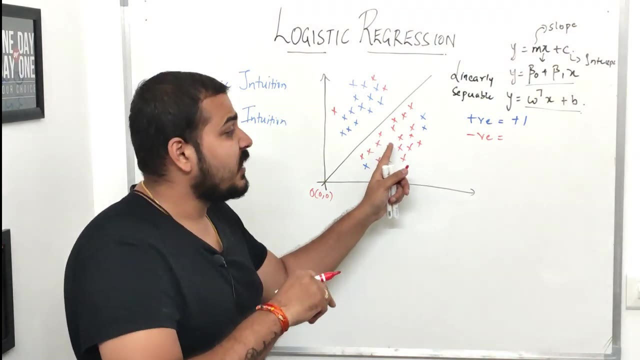 I hope you are easily able to understand this thing, because it is important. guys, This is the major assumption that is actually made in logistic regression: All the positive points is actually denoted as plus 1.. Now, what about the negative points? Now, the negative points, which is this, which is my another class, is not denoted as 0.. 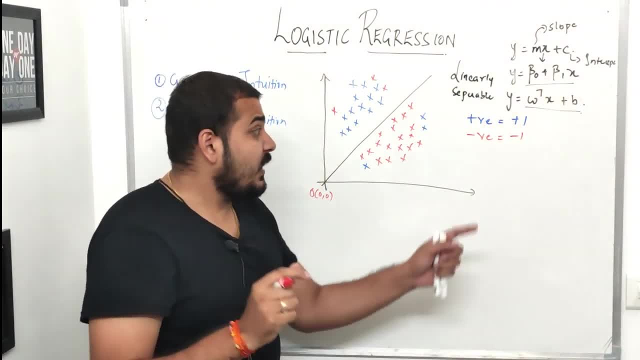 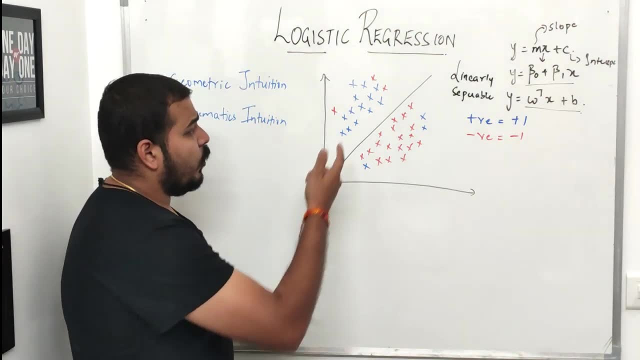 Instead it is denoted as minus 1.. I'll tell you why exactly it is denoted like this. okay, It is pretty much important to understand. Now we know that over here you can see, this best-fit line is passing through the origin, right? 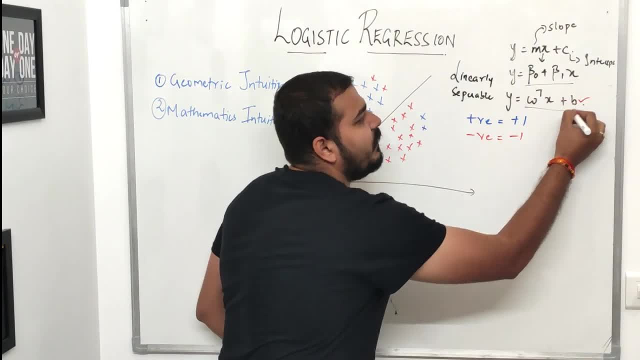 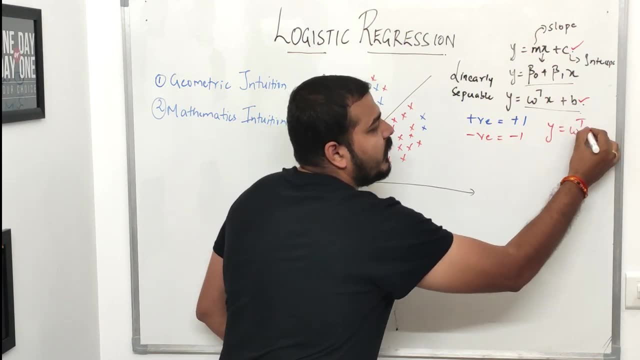 It is passing through the origin, Then I can basically make this B value or the C value as 0, right? So if I make that, it will just be nothing but W multiplied by X, since it is passing through the origin. The intercept is passing through the origin. 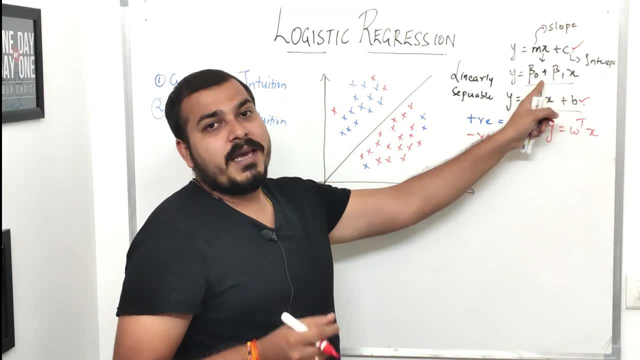 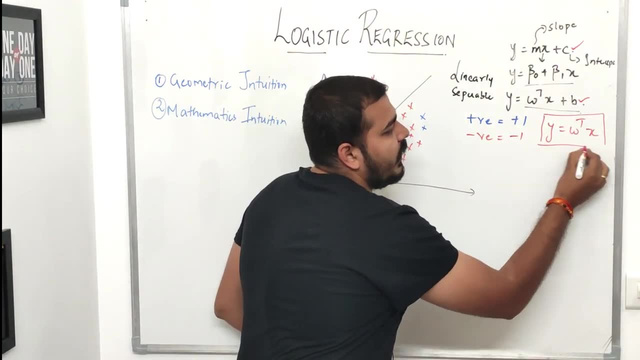 I am basically making this and in this particular case also beta 0 will be actually 0, okay, So when we are doing this now, my equation looks something like this: right Now, my equation basically looks something like this: Now, in this particular case, understand one very, very important thing. 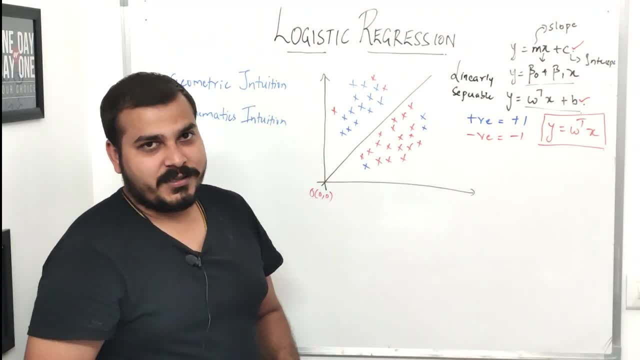 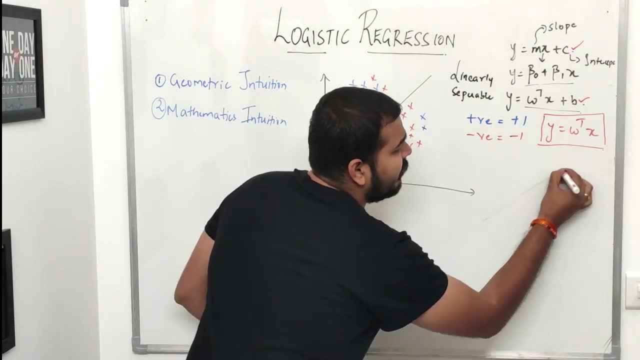 What is this WT of X that you need to understand? Now, I don't know whether you are familiar with linear algebra or not. If I have a straight line which looks like this, okay, Just let me rub it. I don't know, My marker is not working well. 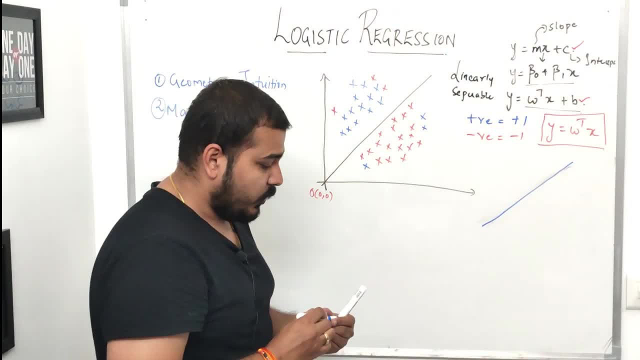 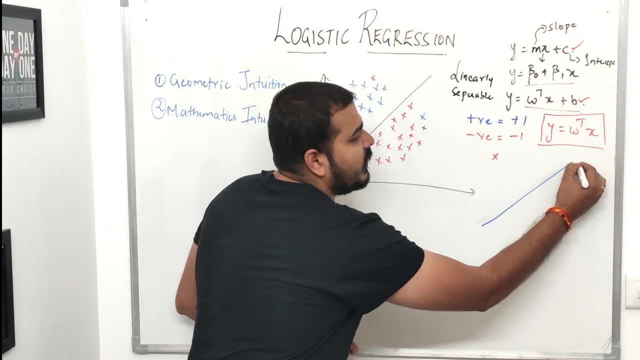 Okay, let me make a straight line like this and suppose: if I have a point somewhere here, okay, If I have a point somewhere here, this is my plane. okay, This is my plane. I can just write it as this is my plane. 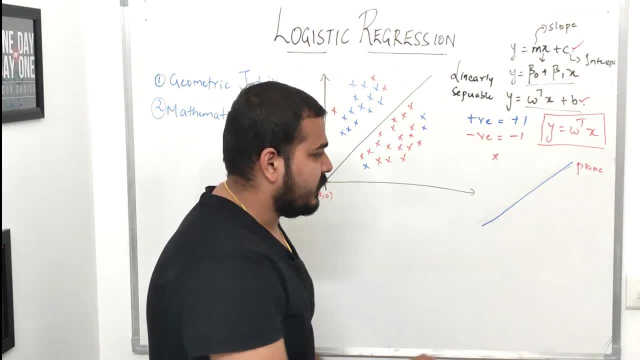 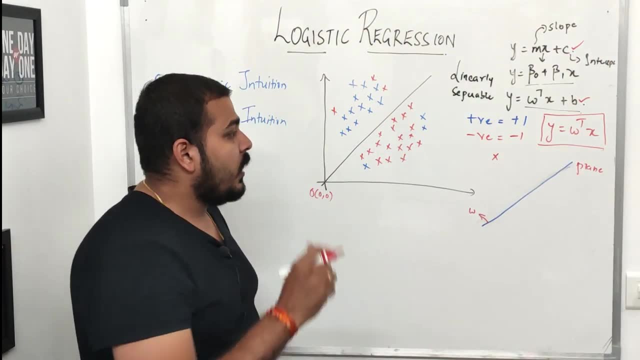 Okay, and with respect to this particular plane, I'll have some coefficients, some W value, right? So I'll have some W value, right. I hope it is pretty much clear. We will have some coefficient value. Now, if I want to find out the distance between this particular point and the plane by the help of linear algebra, 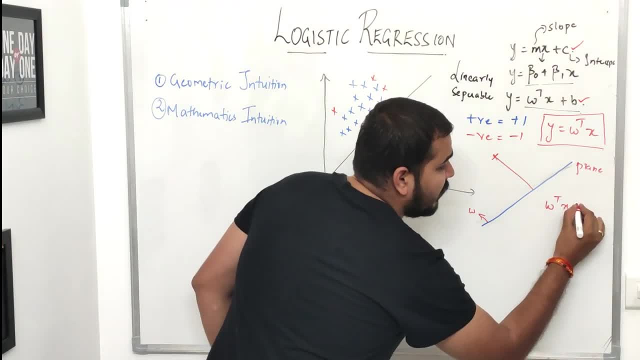 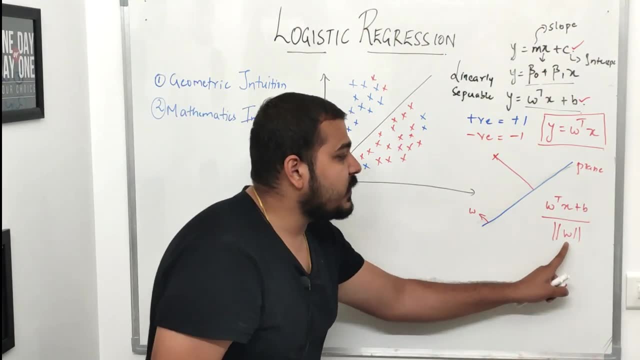 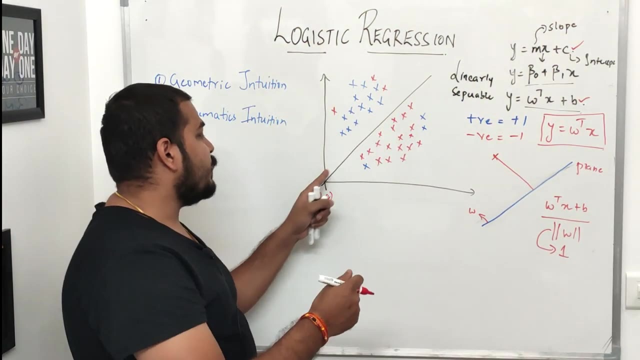 we usually write the equation as WT of X plus B divided by the truth value of W. okay, Now, if we consider this W as a unit vector, this exactly becomes 1, right, And apart from this, since the line is passing through the origin, which I am considering it okay. 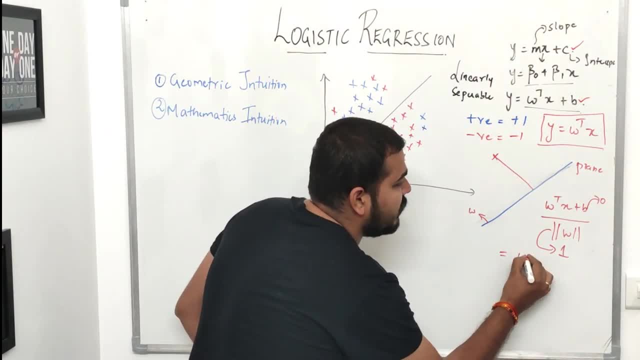 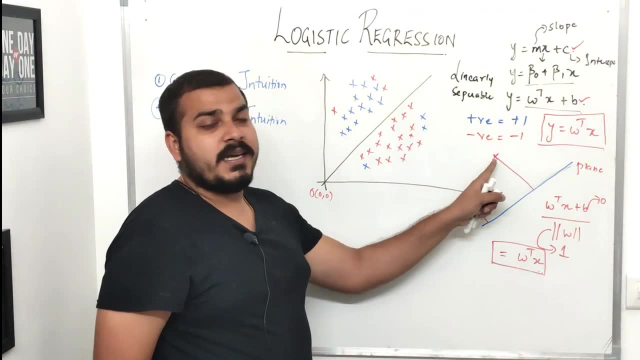 I'm going to make this B value as zero. So this is nothing but WT of X. Now you can say that WT of X is nothing, but it is the distance of this particular point that is my X and this particular plane. 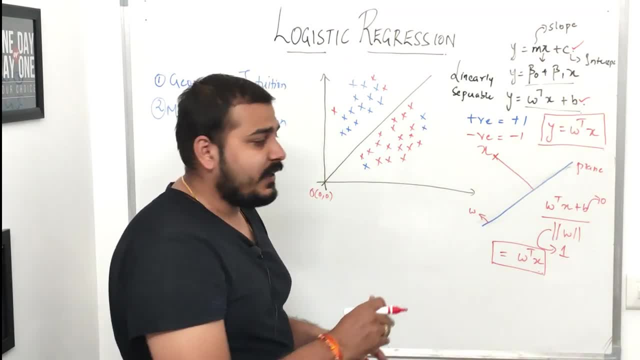 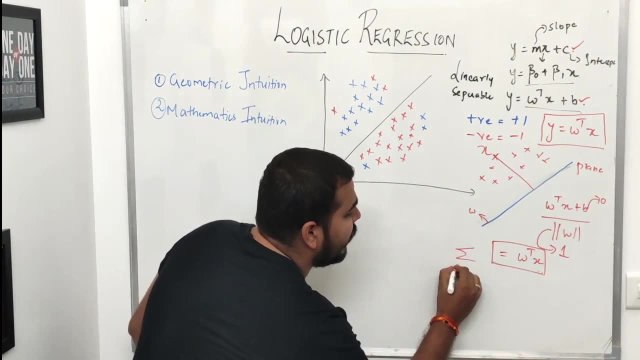 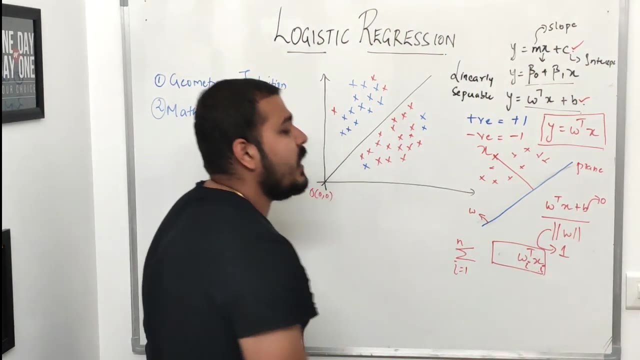 Okay, Now there may be various points over there. right, There may be many number of points like this. if i want to calculate the summation of distance, it will nothing become, then it will just be written as: summation of i is equal to 1 to n. wt of x of i. right wt w of i of t of x of i. 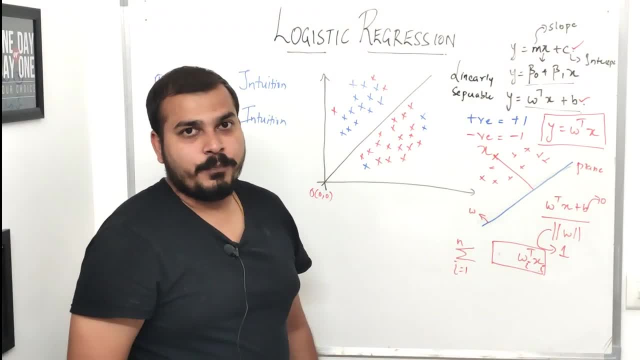 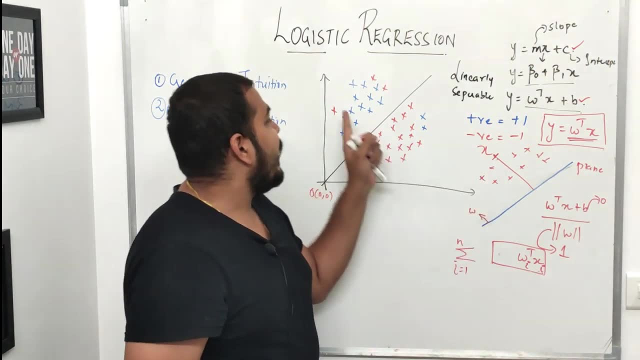 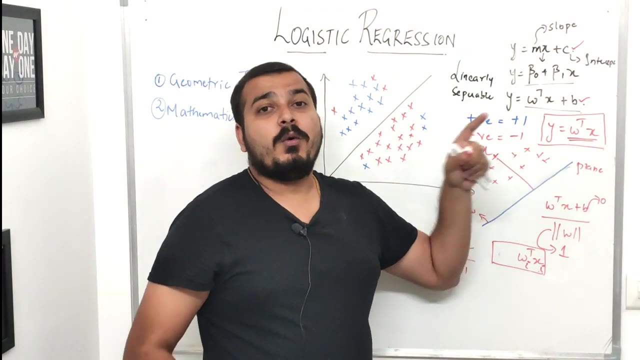 so, like that, we'll be able to find out the summation of this particular value. okay, so instead i can call this: wt of x is nothing but distance between the point, that is, my data points, and this particular plane. okay, so in this specific case, we need to find out a way wherein this w of t? 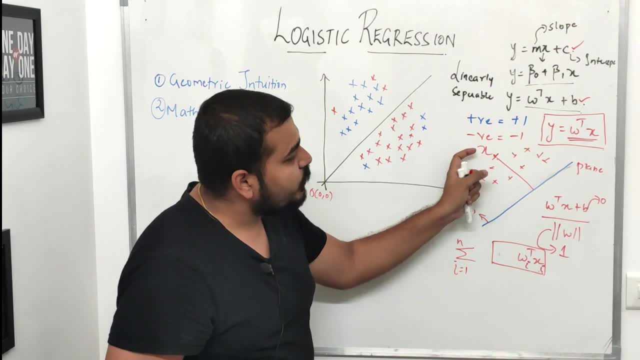 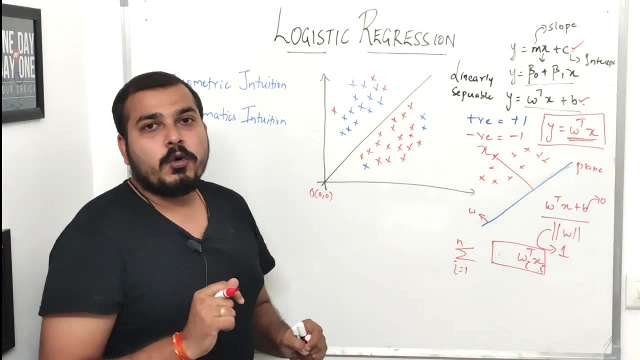 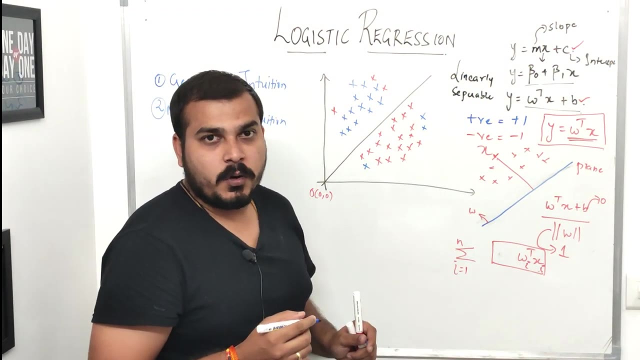 of x is nothing, but it is just this distance between the specific points and the plane. now it will make more sense when i'll be applying over here. okay, now one more point that you need to know. okay, now, suppose guys above this particular plane, if i have this specific points, okay, usually when 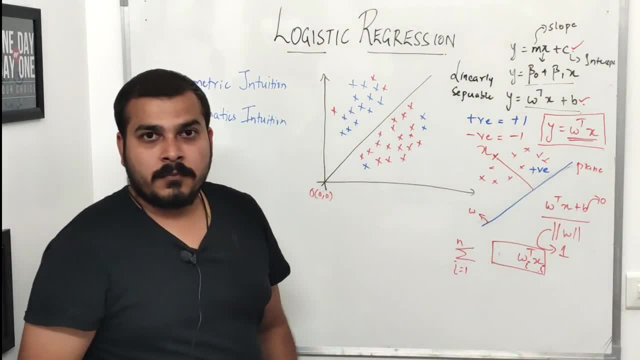 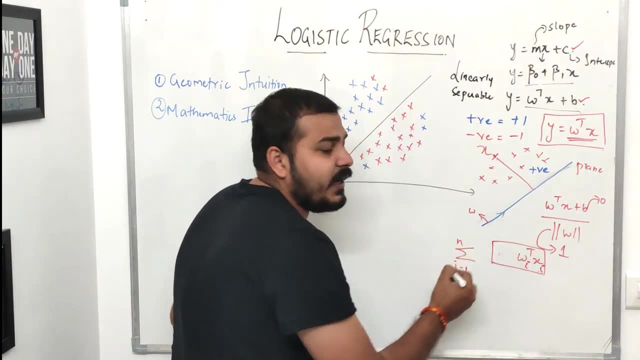 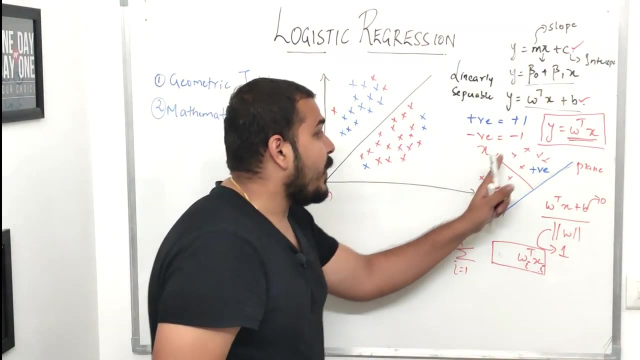 i calculate the distance, it will become positive. now why? because understand, guys, this is my slope and you know that when i'm a positive moving slope, right, if i calculate the derivative, the slope of the derivative is always positive, right? so when i'm applying this particular equation and trying to find out above, above of this, 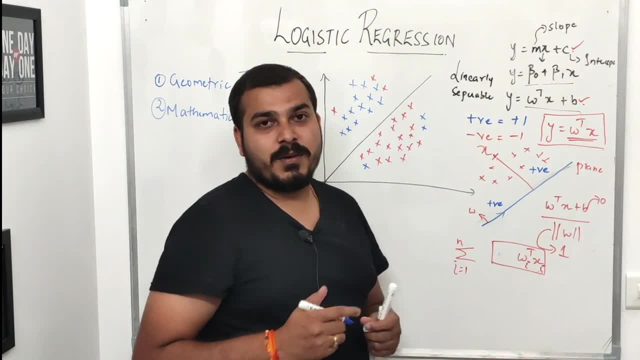 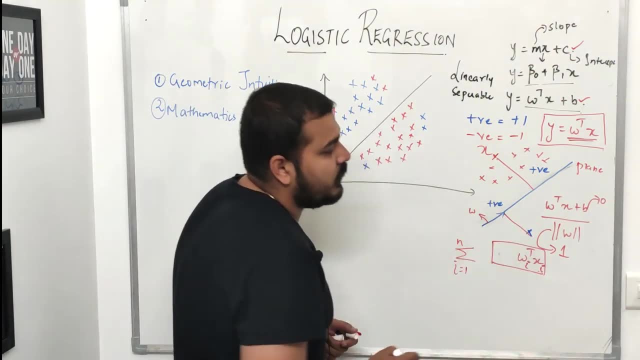 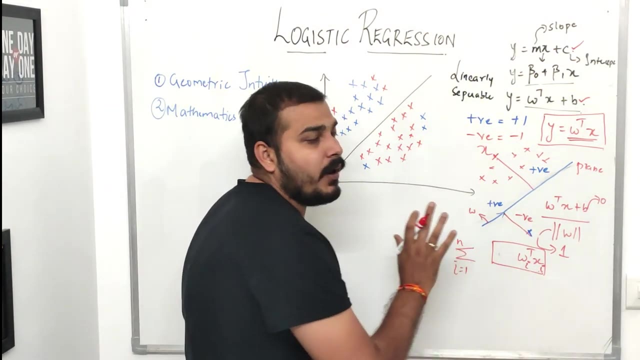 particular plane will always be positive, the distance will always be positive. but suppose, if i have a point somewhere here, if i want to calculate the distance between these two points, that is, this point and this plane, the distance usually becomes negative. okay, so these are the points that you need to remember. okay, in this particular case, again, guys, there is no. 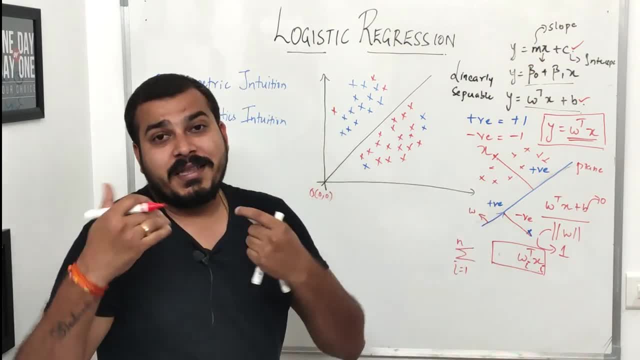 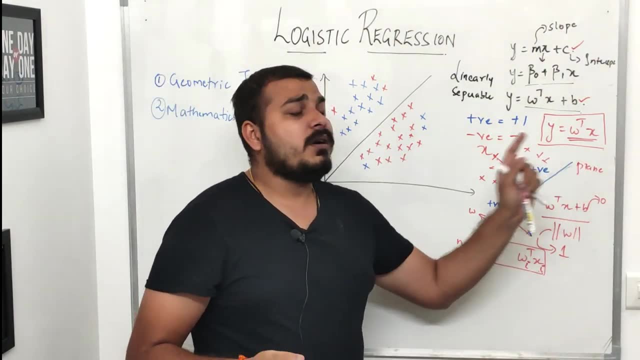 derivation as such required. but understand these are some things that we have already studied in our 12th standard. you know, this is how we actually calculate the distance from a point, from till a plane. okay, if it is above, it is basically positive value. if it is below, it is basically a negative. 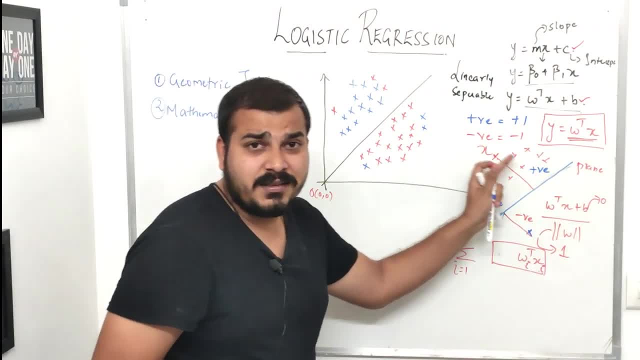 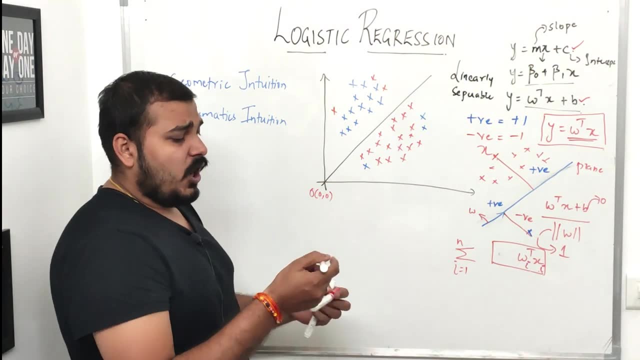 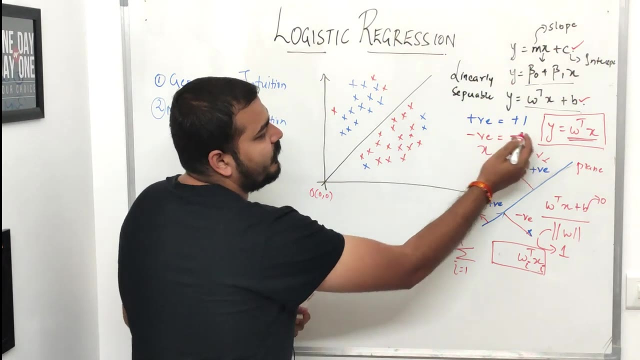 value now, when we have done this, when we have done this. okay, now, just understand one thing, now suppose, understand in this particular case. let me just take case one. okay, over here i've telling, told that there are two points: positive values plus one, negative values minus one. so let me consider: this is my y, okay, y of i, y of i. 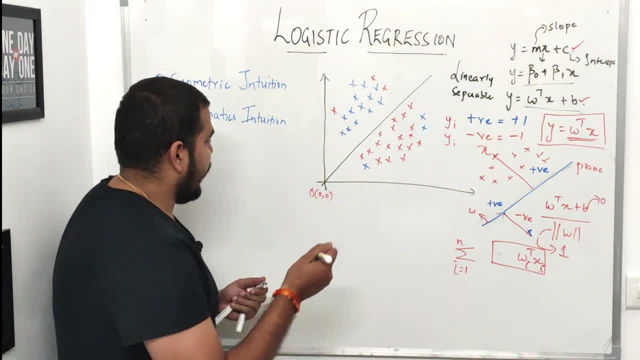 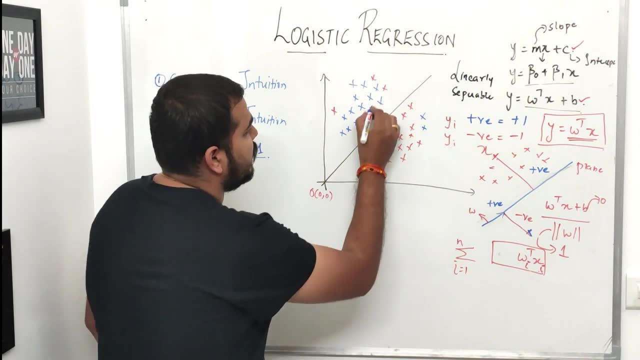 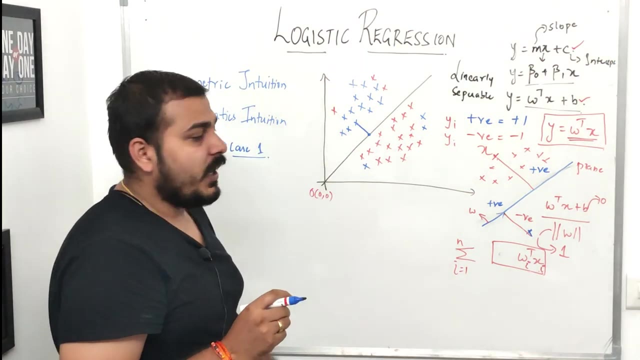 okay, i've just considered it. now, first case, case one, case one: okay, suppose this is my x of i point. okay, this is my x of i point. i want to calculate a distance between this point and this point. okay, i know that this x of y is positive because it is a blue point. okay, so how? 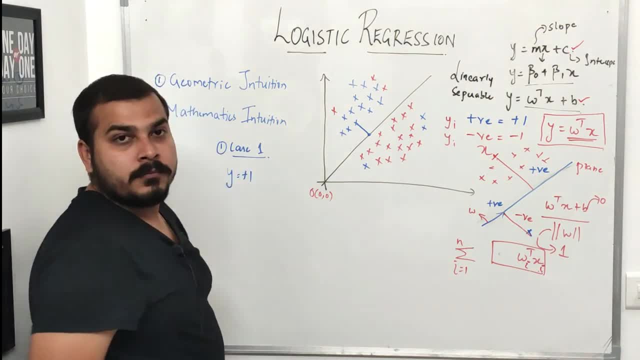 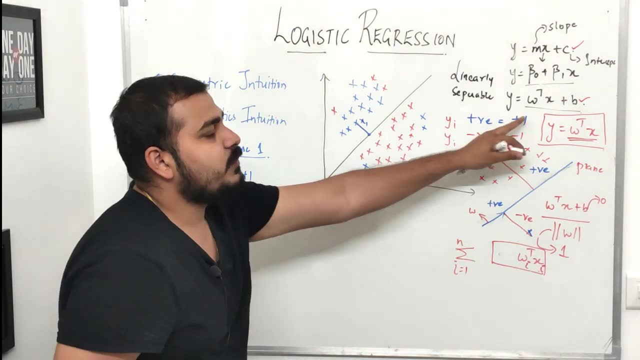 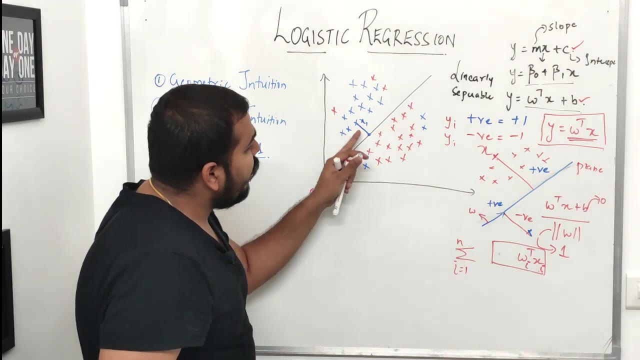 it is denoted. it is denoted as: y is equal to plus one. okay, so i'm considering this y of one. suppose this is my x of one point. i know the value of y of one. it is basically positive. okay, so now over here. y of one is positive. now, if i want to calculate the distance between this point and this point, 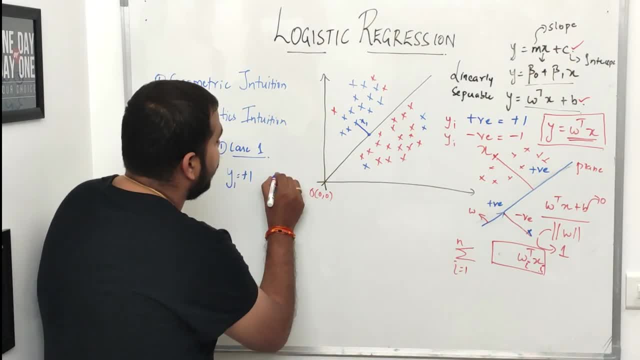 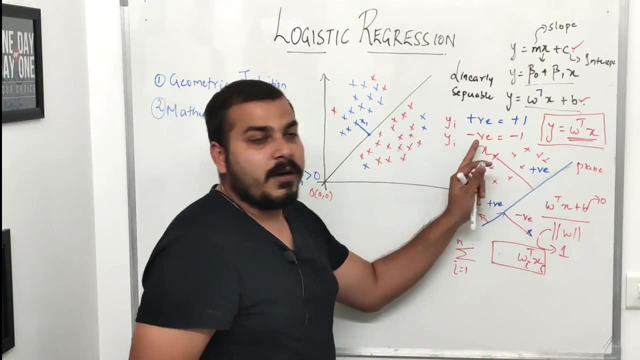 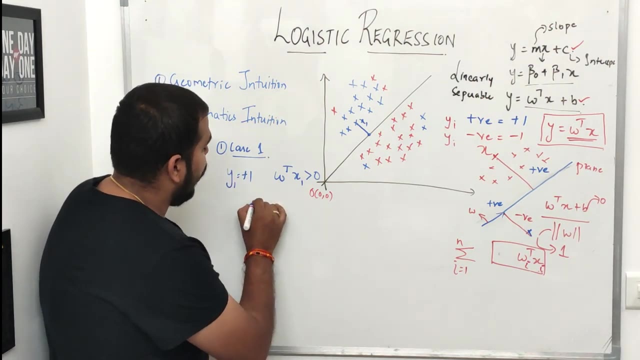 to calculate the distance between this two. point then what i'll get. i'll get nothing but w, t of x, of one is nothing, but it will be greater than zero, since i told you that above the plane the distance is positive. okay, so this is my case one. now what i do is that i will apply a formula. 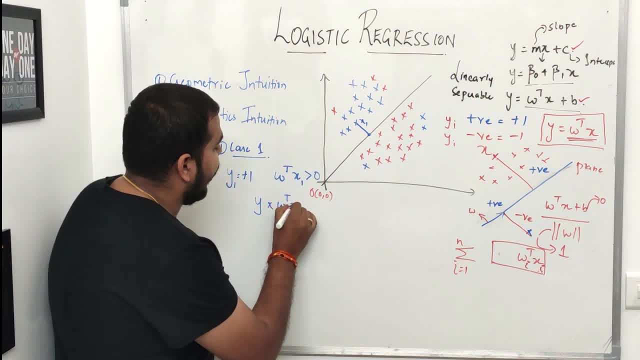 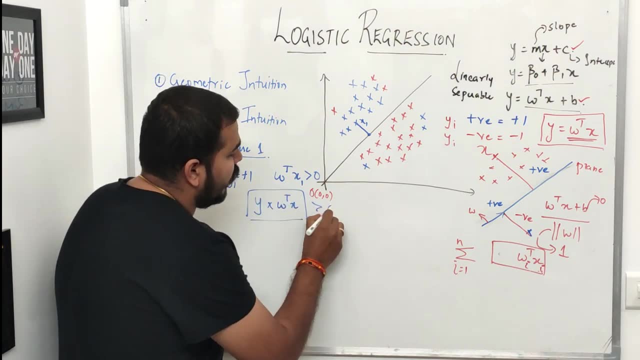 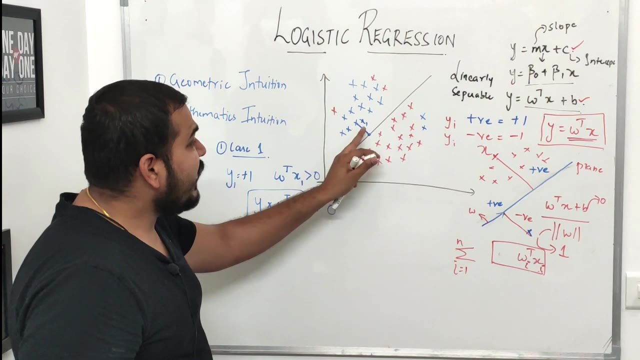 wherein i will multiply y multiplied by w t of x. understand this particular point, guys. when i multiply y multiplied by w t of x, it is going to become greater than zero. that basically indicates that if i have this kind of scenario, it is getting easily classified, right? 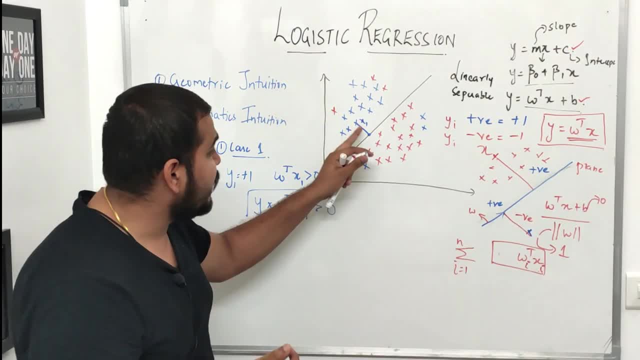 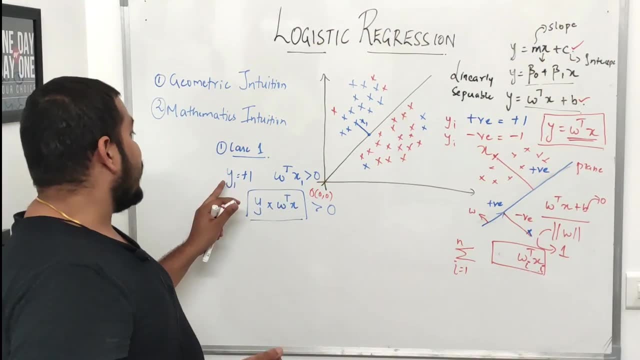 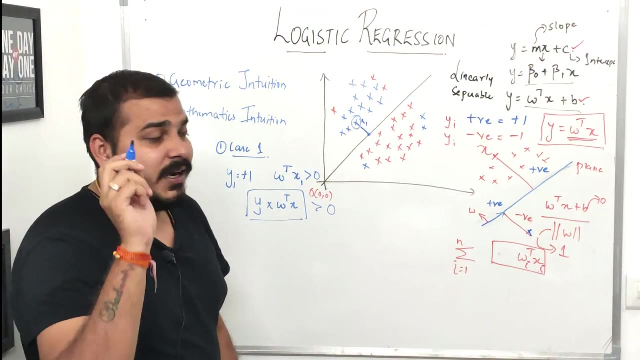 so whenever my y value and w t of x- that is, the distance between the plane- is positive, right, i'm getting a positive value. and i know, since i'm getting a positive value, this y of i is properly classified. this is my positive point, right? i hope you're understanding this. okay, now understand. 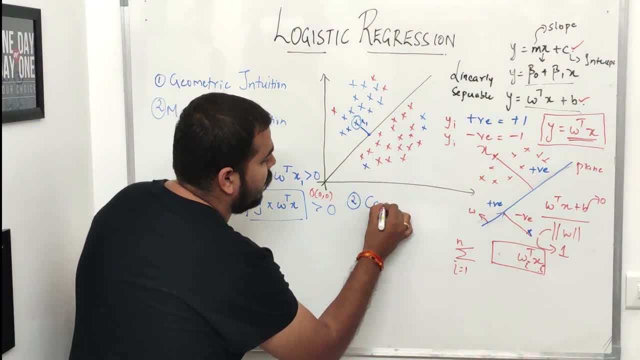 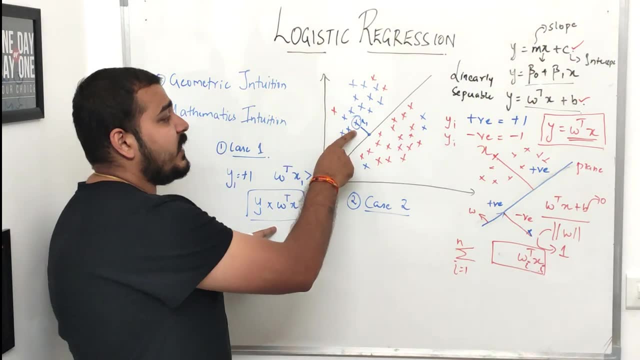 about the case two. so i'm going to discuss about my case two now. in case two, let's say i'm going to take a negative point and always remember when i'm getting this value. in this case that basically means the classification has happened correctly. okay, that that has happened correctly over here. 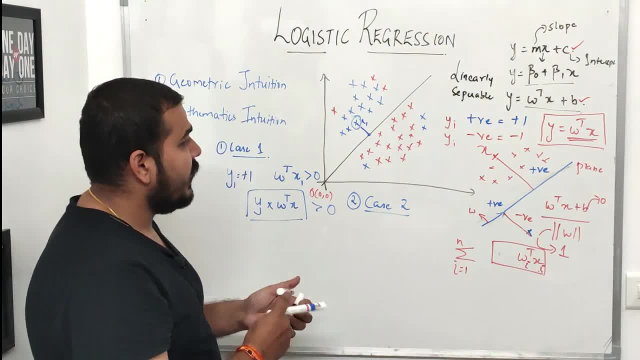 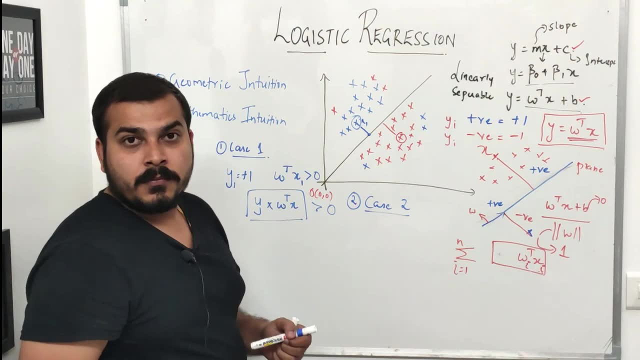 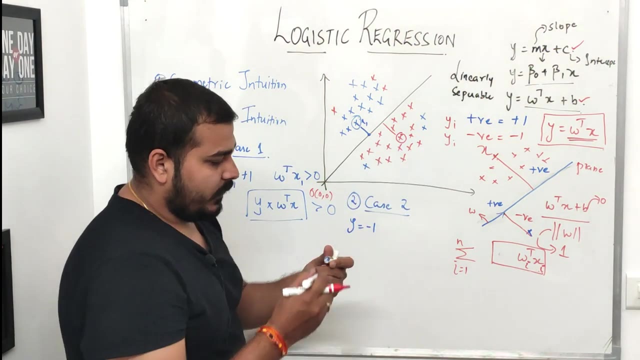 okay, now the second case. what i'm going to define over here is that suppose let me consider this particular point and i'm going to find out the distance between this. okay, now, in this particular case, i know what will be my y, i value my y, i value will be minus one, since this is negative. 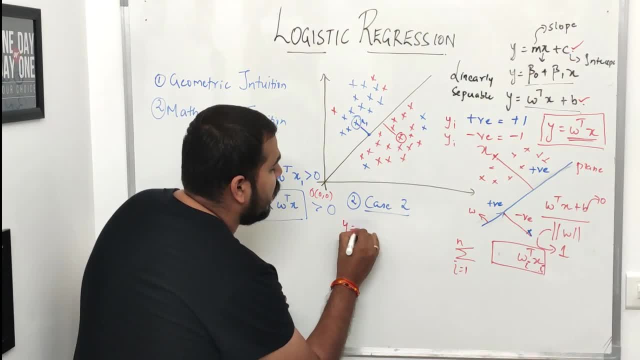 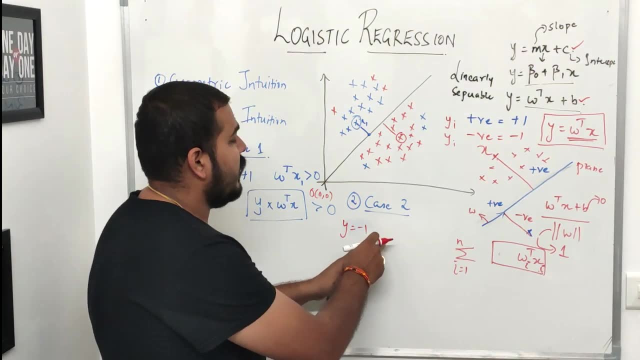 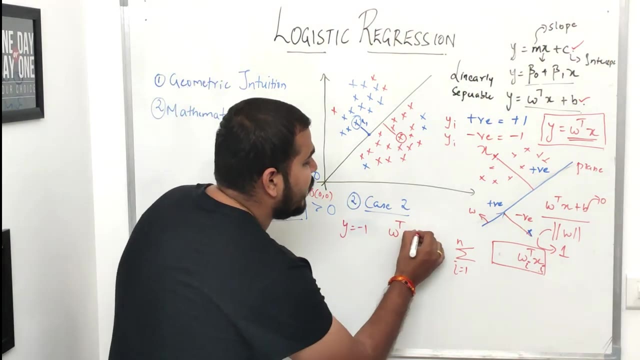 let me just write it in red color so that you don't get confused. this is a negative value and we have initialized negative value as minus one. okay, now, when we have y is equal to minus one. here you can actually see that when i'm going to compute w t of x, in this particular case it is going to become less than zero, since 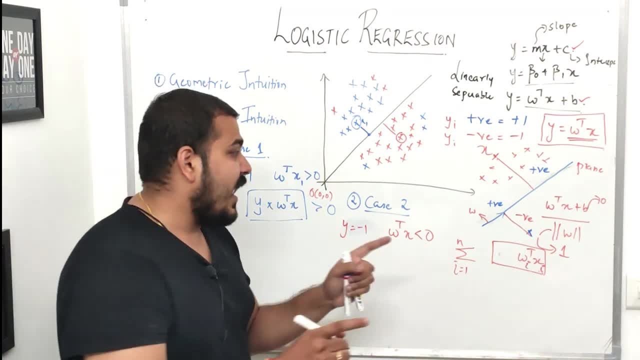 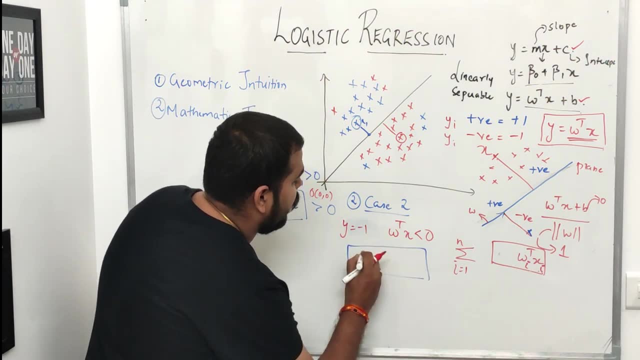 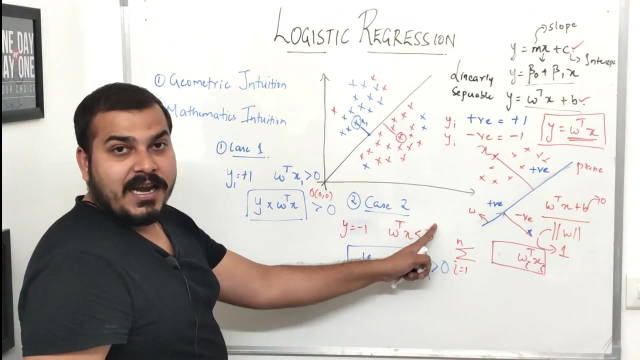 this is going to give me a negative value. okay, now, when i have this negative value, now again, what i'll do? i'll do the multiplication of this two. so when i'm doing the multiplication of this two, y multiplied by w, t of x, it will be greater than zero because, understand, this is a negative value, this is a. 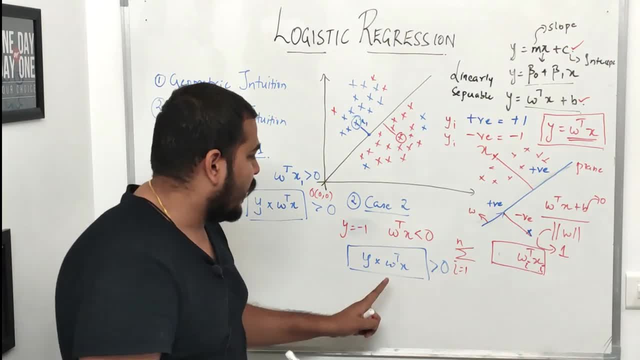 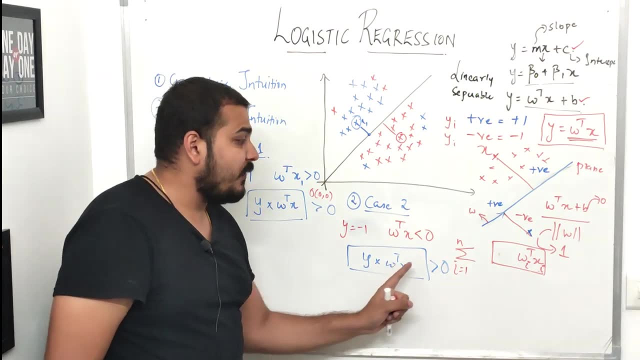 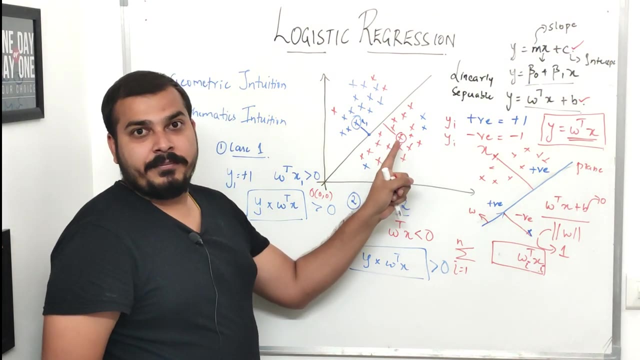 negative value. negative value multiplied by negative value will be a positive value. now understand one more thing again here. since the summation, since the multiplication of this particular value is greater than zero, at that time what is happening? this particular point is getting classified correctly. okay, because we are able to classify this point. okay, since this 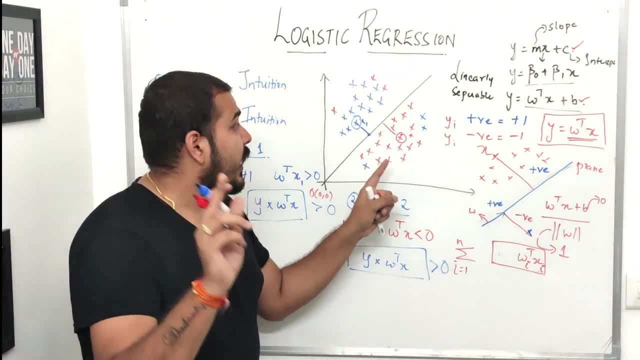 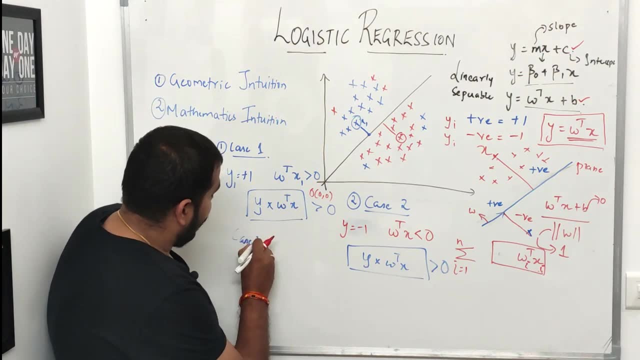 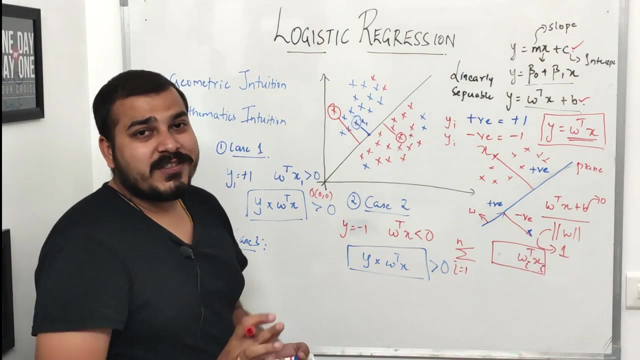 particular point is minus one. understand in this particular way, guys, okay, now suppose let me take another case, my case three. okay, suppose i i'll just define my case three over here. let me consider this specific point and i want to compute the distance between this and i want to see that, whether this is properly classified or not, now in this particular case, 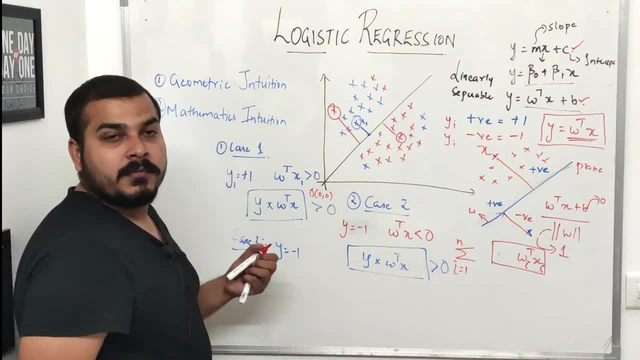 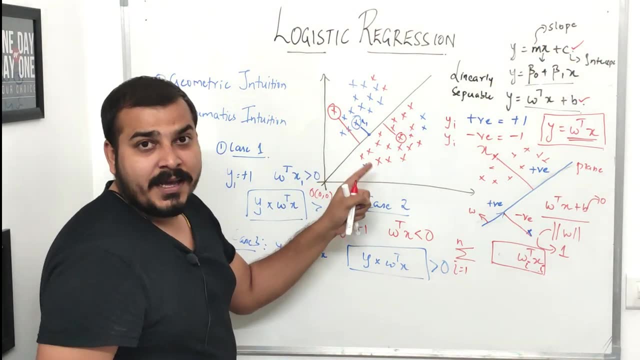 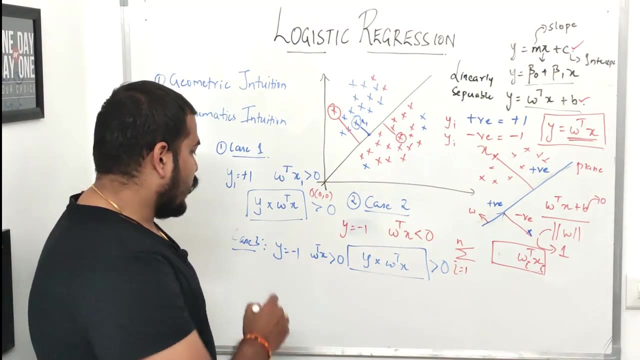 what will be my y value? my y value will be minus one right now. what about the distance w t of x, distance of this particular point in the plane? it will be positive because i understand above the plane, it is positive, so here it will be greater than zero, right? so if i multiply y, multiplied by w t of x, this particular value, considering this, 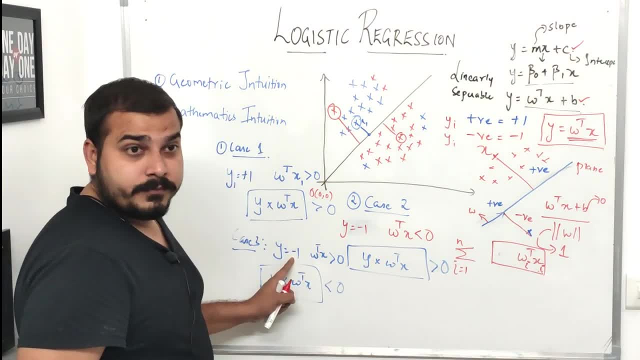 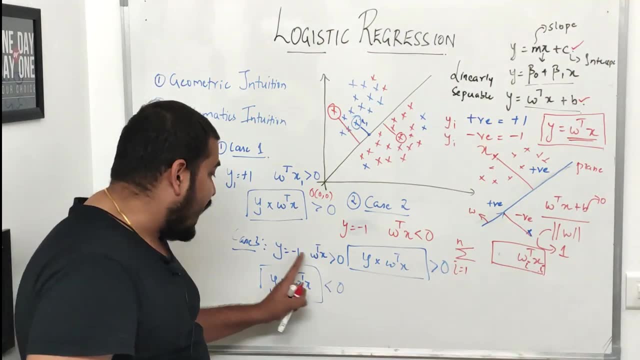 will be less than zero, because i have minus one over here, and this is a positive value. negative value into a positive value will be less than zero. now, when we have this particular value less than zero, at that time what will happen? understand this thing, guys, this value. 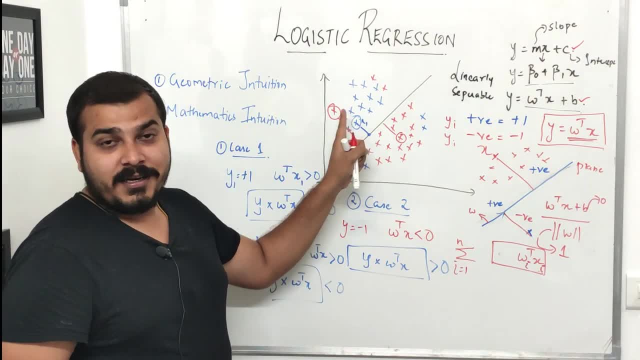 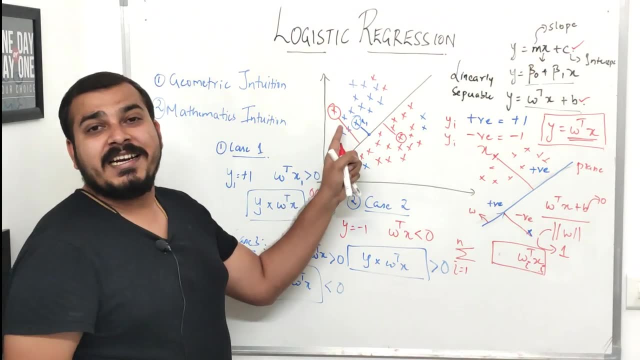 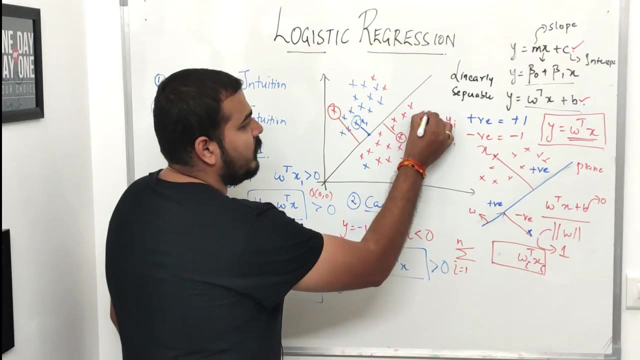 you can see that this red point is incorrectly classified right now. this basically indicates that whenever you do this multiplication of y and w, t of x, if you are getting a negative value, that basically indicates that this is not a correctly classified point. okay, take this particular example now. one more example can be this: if i'm trying to compute the distance, 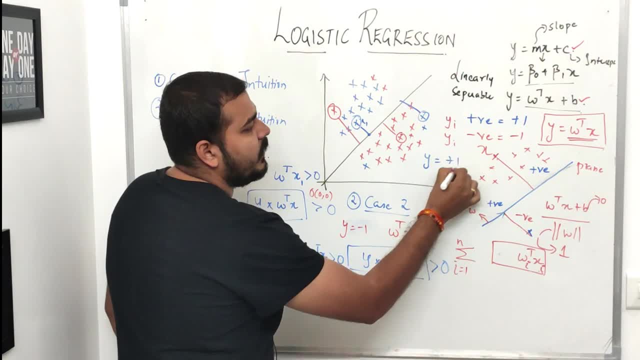 first of all, my y value will be: uh, this will be plus one right now. if i calculate w t of x, this distance below the plane is negative, so this will be a negative value. if i multiply two, this will be a negative value. now, when this is again a negative value. this is incorrectly. 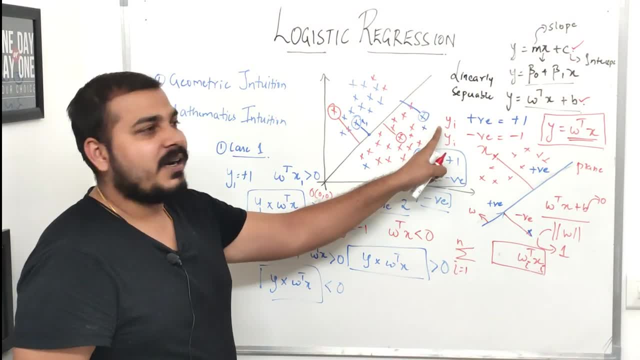 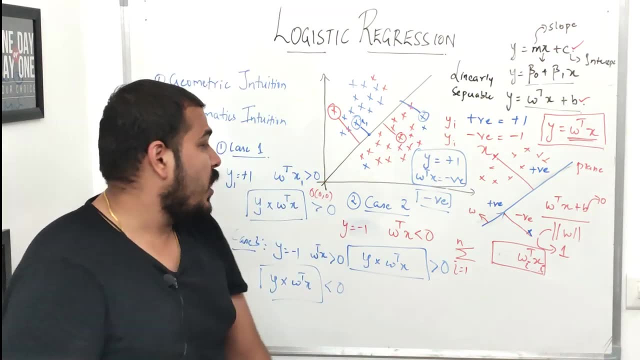 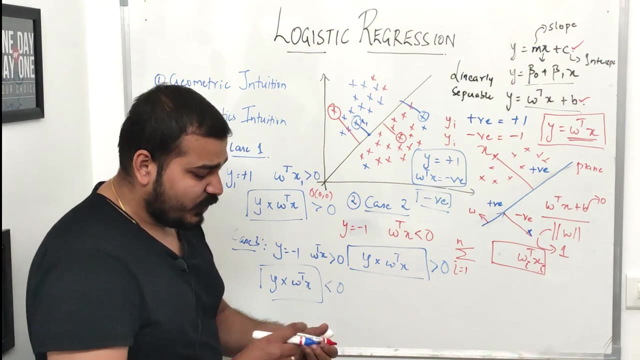 classified because this blue point does not belong over here, but since we have this kind of point, this will get incorrectly classified. now, the most important thing that you need to note down from all these cases is that right. what you have to note down from these cases is that i'm just going to write a very, very simple thing in front of you is that 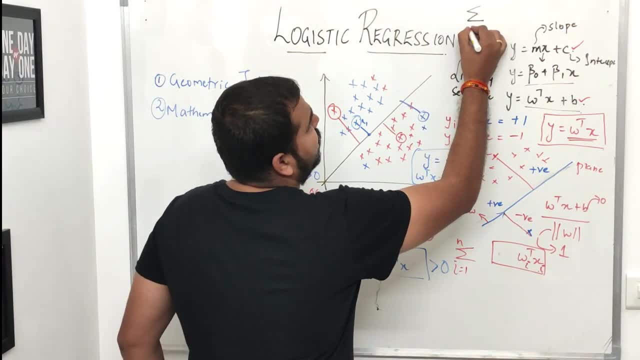 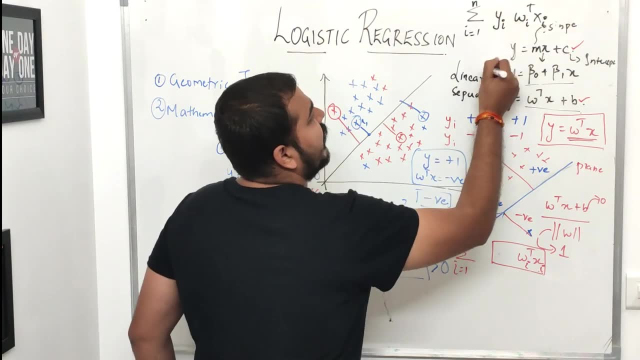 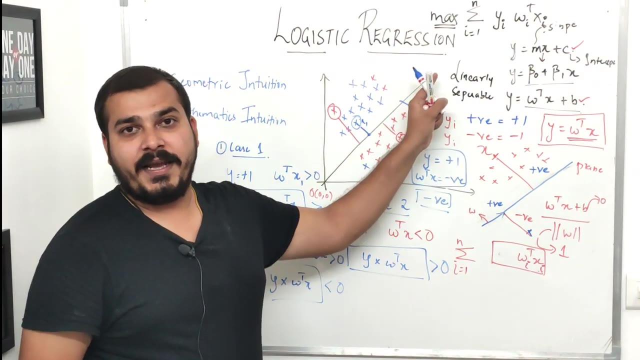 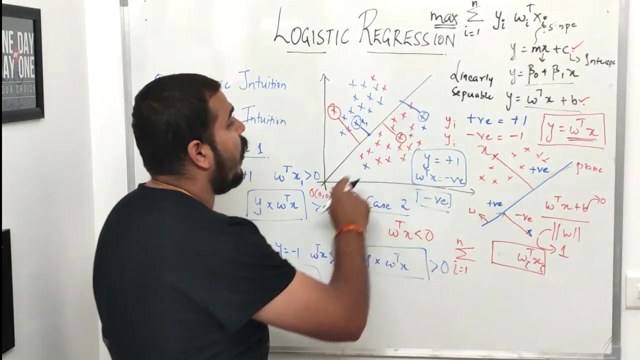 our cost function right, it will be something like this: i is equal to one to n. w of i multiplied by x of i should be maximum as possible. if i want to create this straight line, the best fit line, which linearly separates to this particular points, i have to make sure that the summation of 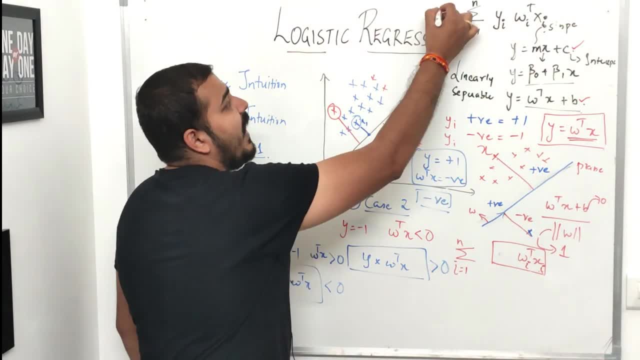 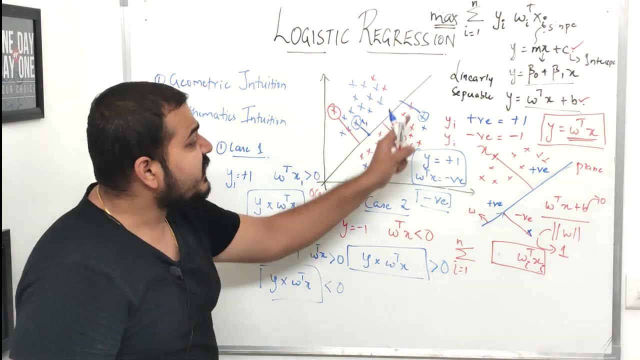 all the points, along with the distance, should be maximum. right, because this indicates when it is greater than zero, all the time when it is greater than zero, it is correctly classifying all the points, both the positive and the negative points. but if the value of the multiplication of 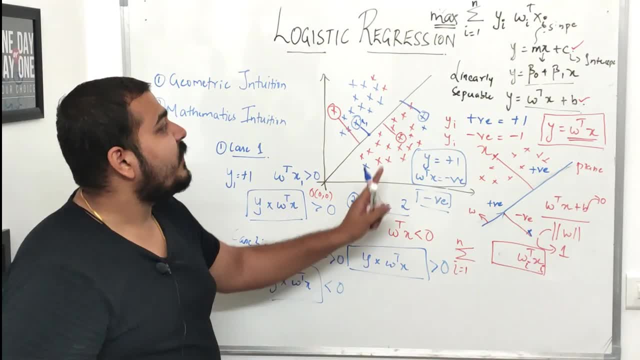 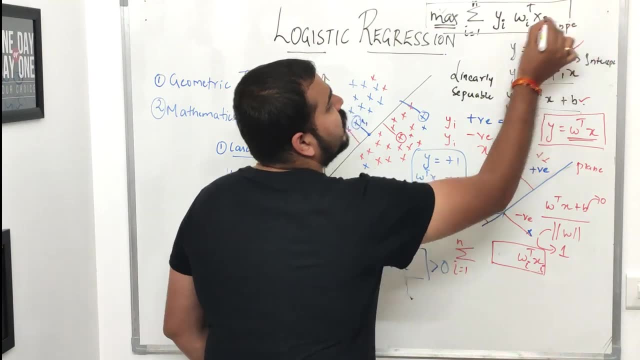 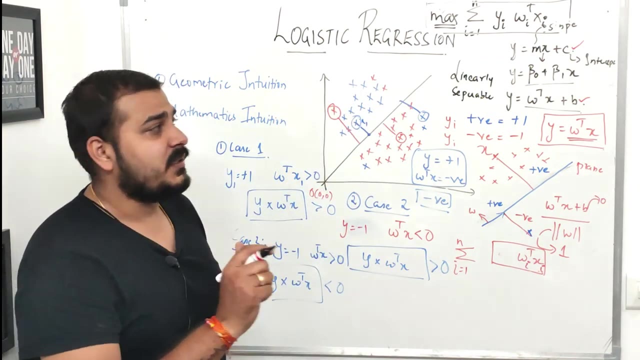 w and w. t of x is less than zero. it is not classifying the points properly. so this is basically my cost function and, considering this particular cost function, we have to focus on creating this particular best fit line. now in this note one thing, guys: our w of i. 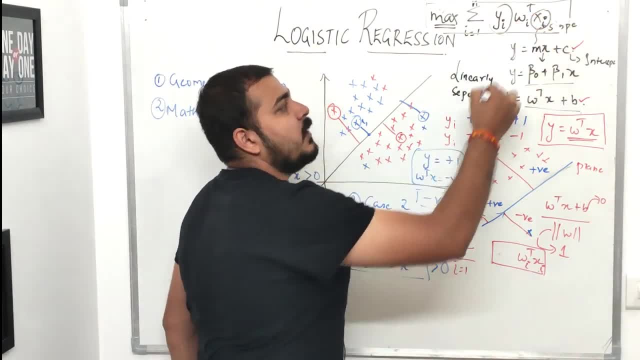 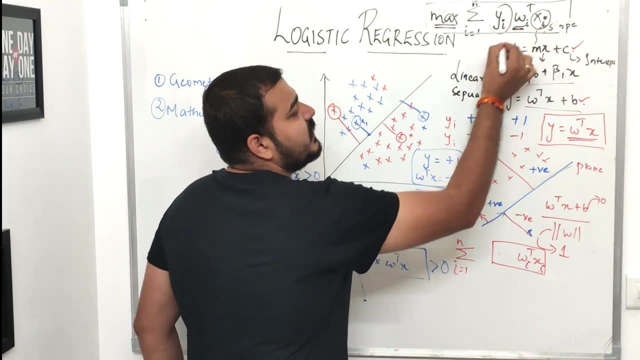 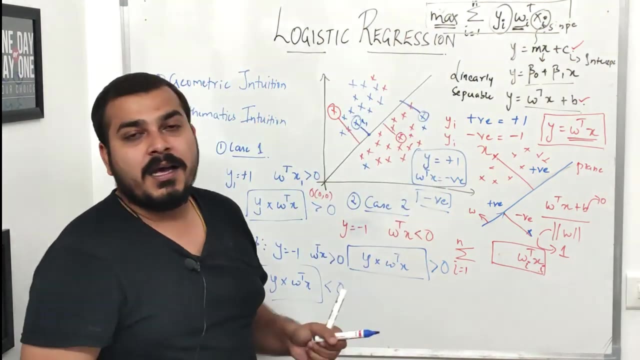 is given, our x of i is given. the only thing, the only parameter that we should update, is nothing but w of i, and this w of i is actually our coefficients. i can say w of i, i can say beta. okay, if i say beta, beta, beta of t, like this, i can also say beta, t of x of i, right here. 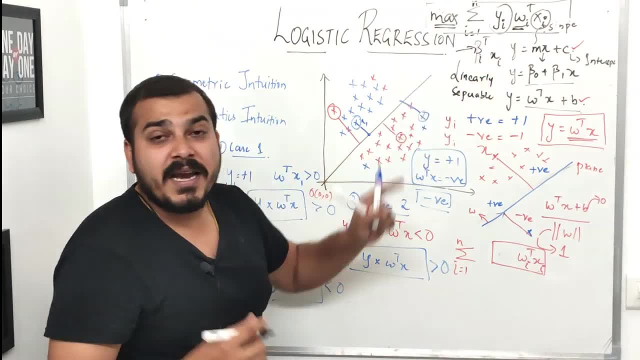 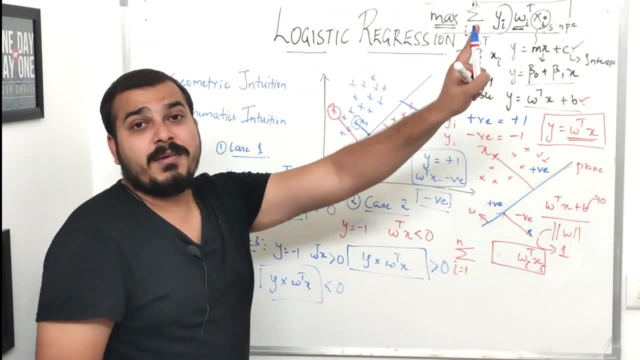 i just have to update this weight. i can say: update this coefficient unless and until i get the maximum of the summation of this weight right. here i can say: i can say this coefficient right when i'm getting the maximum summation of all the points that particular line will specify. 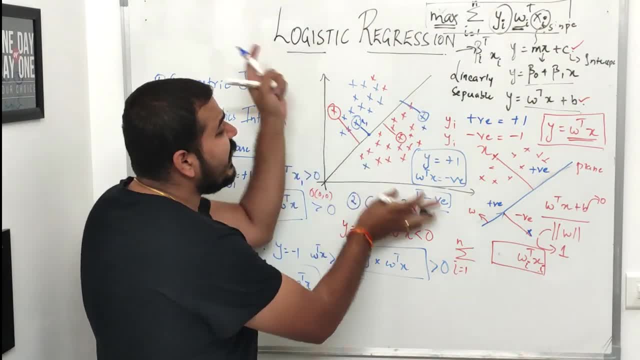 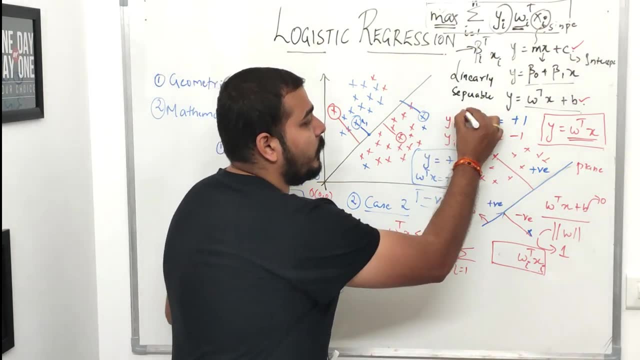 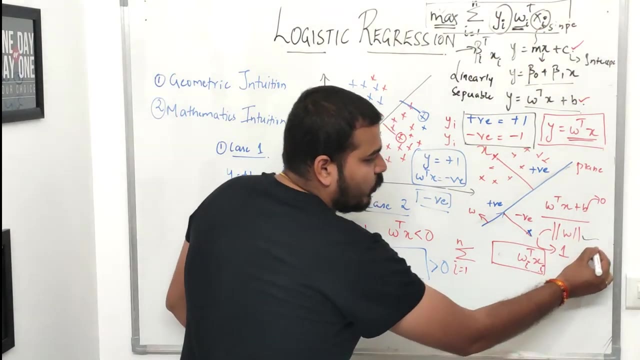 your best fit point, that, sorry, best fit line that linearly classifies both the classification values over here. and remember, this is the most important thing- the positive value is taken as plus one, the negative value is taken as minus one. and remember, this is a unit vector, as i told you. 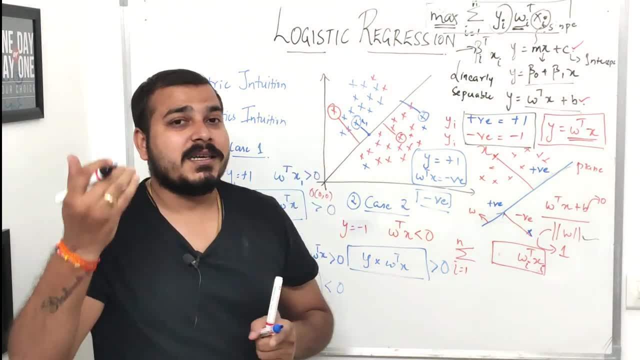 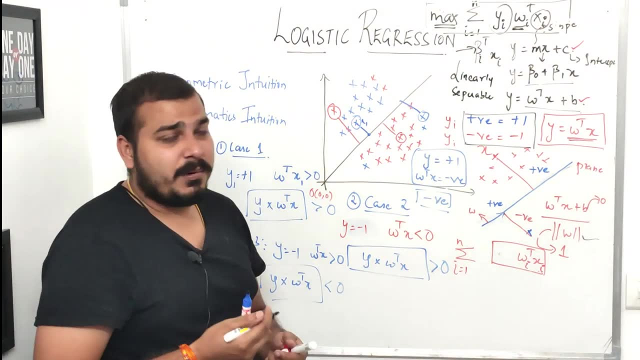 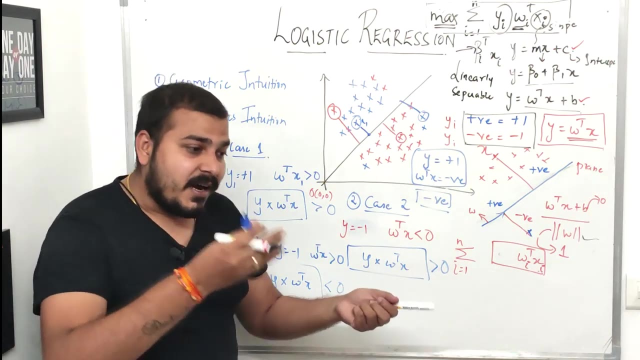 and by this this is how a logistic regression actually works. right, pretty much simple, guys understand. one more thing i'll just revise and give give you an idea about it, and i've referred many, many materials to understand this. you know, when i started learning logistic regression, my 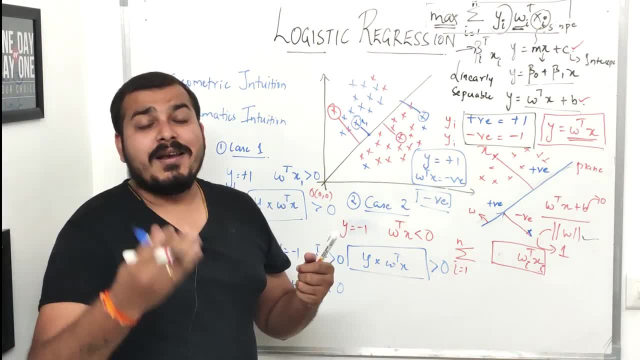 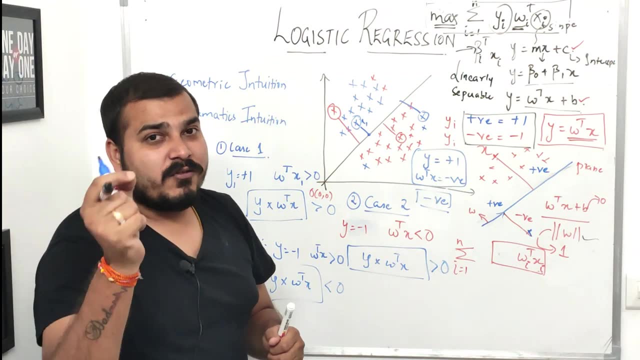 understanding was completely different. then, as time moved on, i learned more, new, new things. then i got to know the proper algorithm, how it actually works, but still we have not come to a sigmoid function. that will try to understand just after this. but the main aim is that, guys, this is my cost function. this. 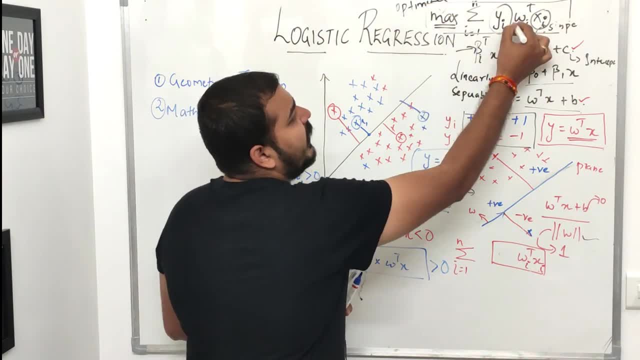 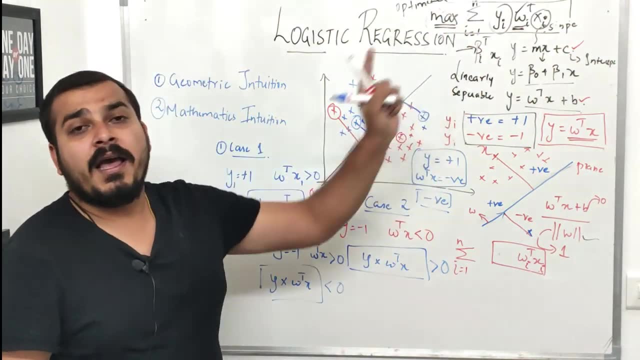 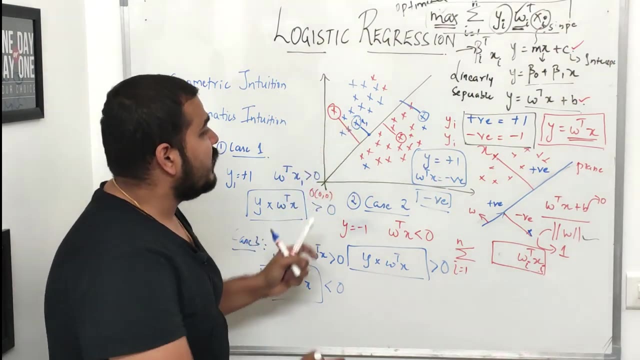 is my optimizer- you can also say it as optimizer- and we need to update this w unless and until we should get this maximum value, and i'm doing the summation of y of i and all the distance between the plane and the points. now, when i'm doing this, when i'm doing this till then this particular line. 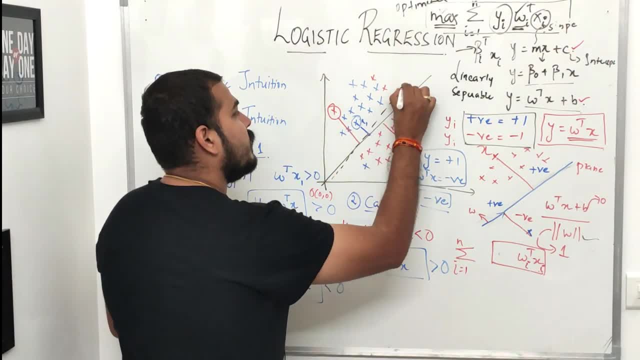 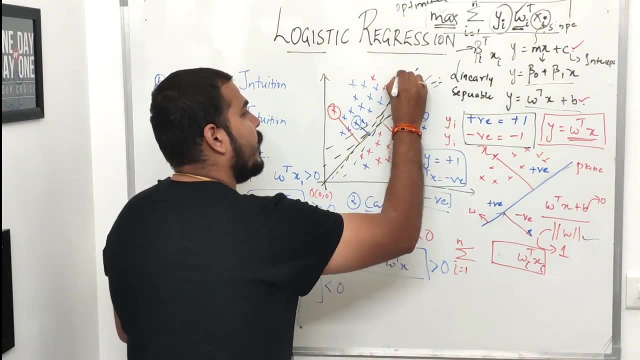 is going to get updated. see, i can have another line which looks like this. i have. i can have another line which looks like this. i can have another line which looks like this, but which is the best fit line? which is the best fit line? that classifies this point? that is a positive and the negative point. 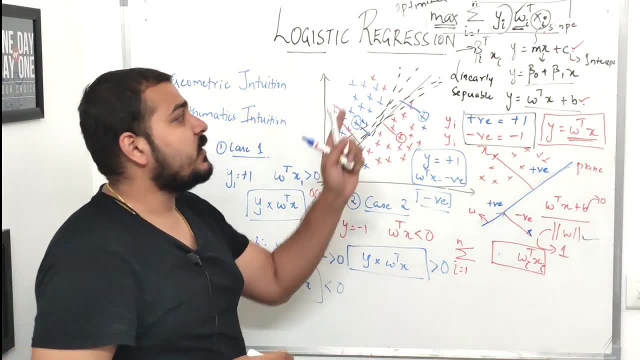 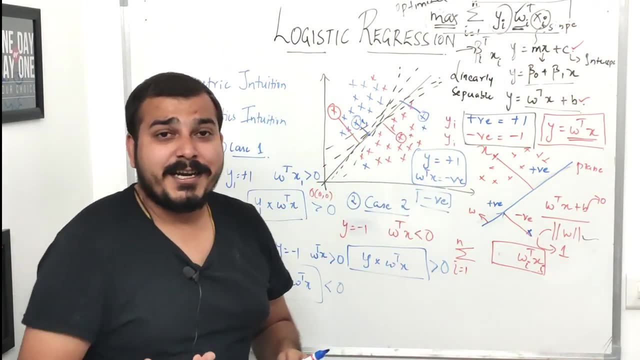 whichever has this maximum summation value, maximum summation of product of y of i with w of i, t of xa, and that is why y of i is basically our training data set. right, we have all our data points like that and, considering that we will be able to get that particular solution and we will. 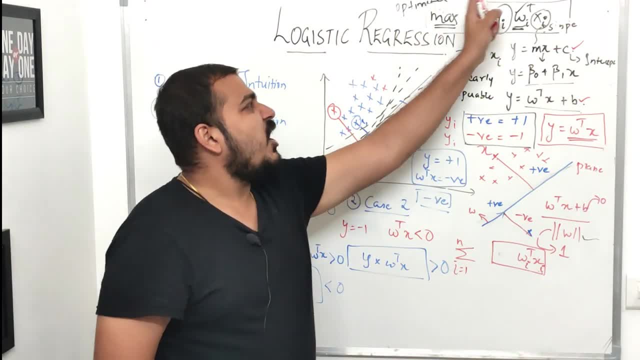 be able to get the best fit line, but still, this is not exactly what we are trying to make. perfect, right, but still this is not exactly what we are trying to make. perfect, but still, this is not exactly exactly the optimizer. there is some more thing that needs to be considered. what i'm going to do, 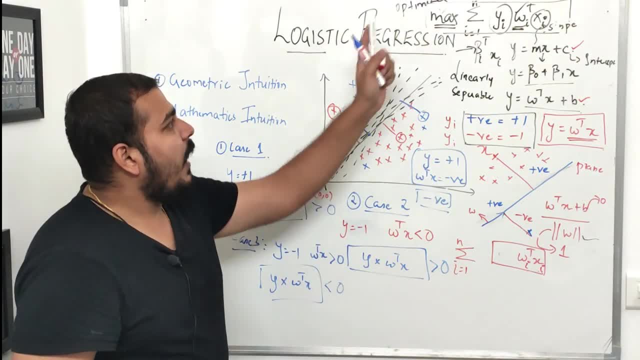 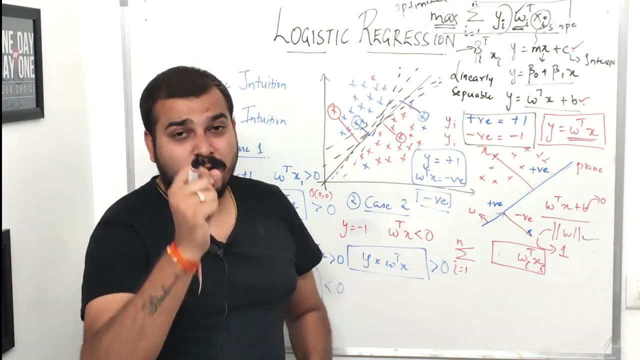 i'm just going to quickly rub this and make you understand, after this equation, what we should exactly do, how this equation will actually get modified and what is this sigmoid function that also we need to understand. so let us continue, guys over here, we have already found out that. 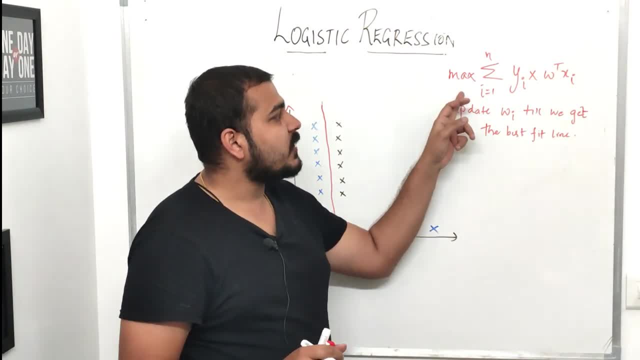 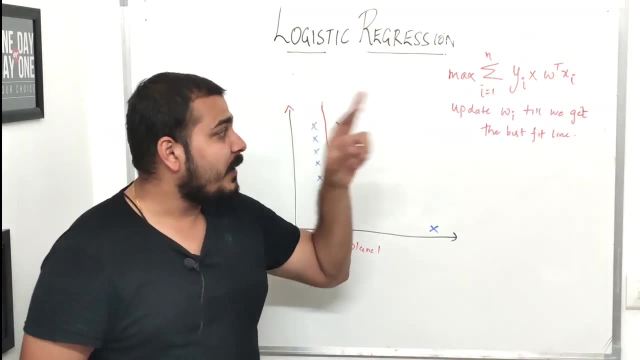 the main aim in logistic regression is actually to find out: max of summation of i is equal to 1 to n w of i multiplied by wt of x of i and this particular value based on the updation of weight, which is giving the maximum value that will actually be used to create the best fit line. 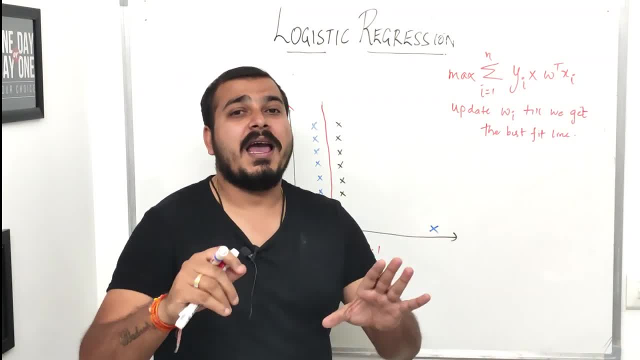 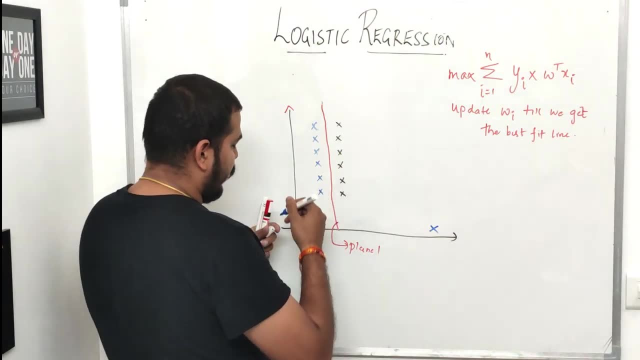 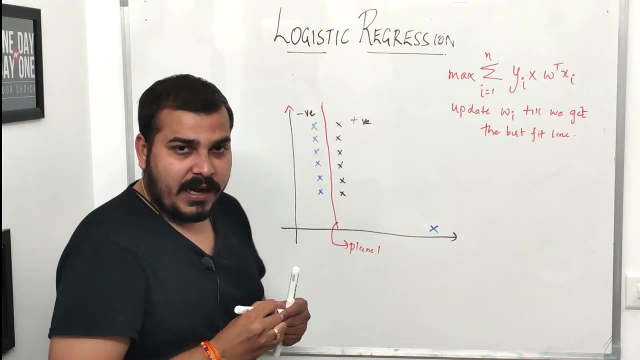 now understand one thing, guys: what will happen if we have some outliers in logistic regression? now suppose i have these two data points. okay, let me consider this: black points are my- uh- positive points and this blue points are my negative points. and uh, just by normalization of this particular value, i will be able to find out what is the best fit line. 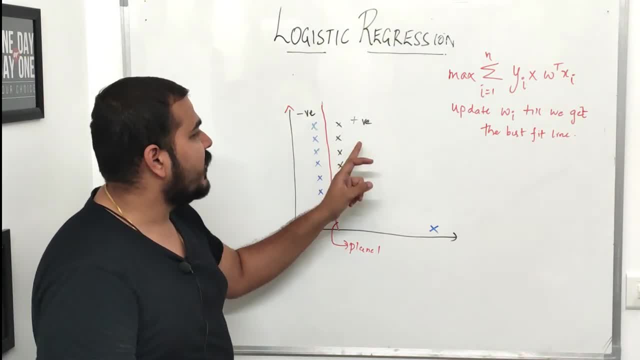 and i will be able to find out what is the best fit line. and i will be able to find out what is the best fit line, normal, seeing that we'll consider that, okay, this is our plane. that is actually dividing this- positive and negative points. now understand one thing, guys: there is an outlier. that basically 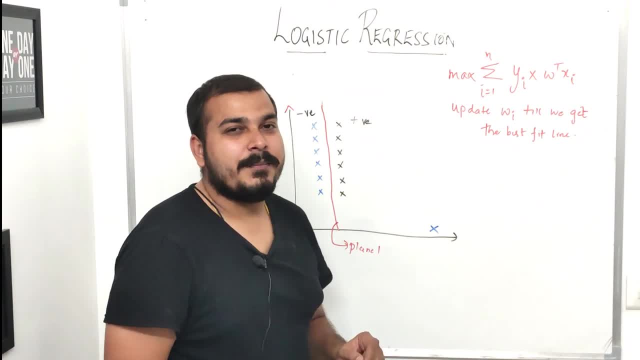 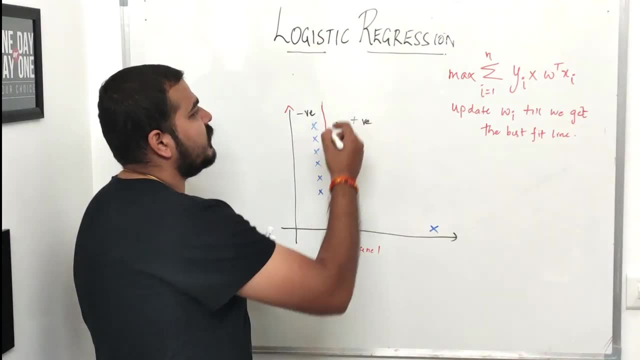 means this particular point is somewhere populated over here, and this is basically my outlier now. what i told is that we need to find out the summation of y of i, wt of x of i, and remember: the positive points is basically given as plus one. the negative point is basically given as minus one. okay now. 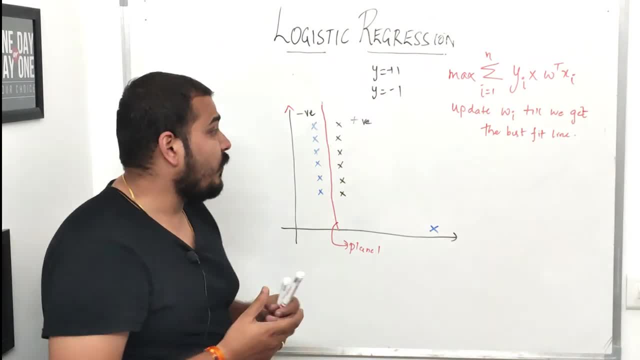 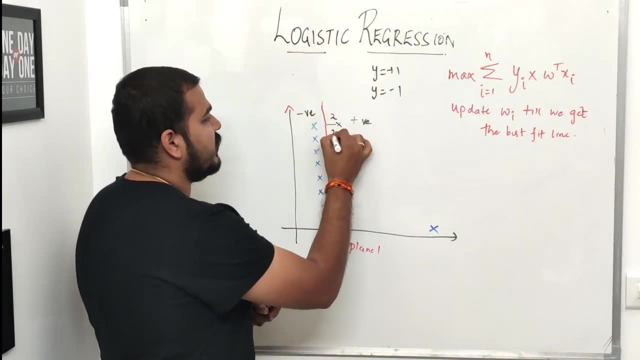 considering this particular thing. guys, what we will now find out is that whenever i'm trying to find out a distance, and let me consider that this all distance are somewhere around two. okay, so this distance is two, two, two, two, two, two right, and again this distance is again two, two, two, suppose. 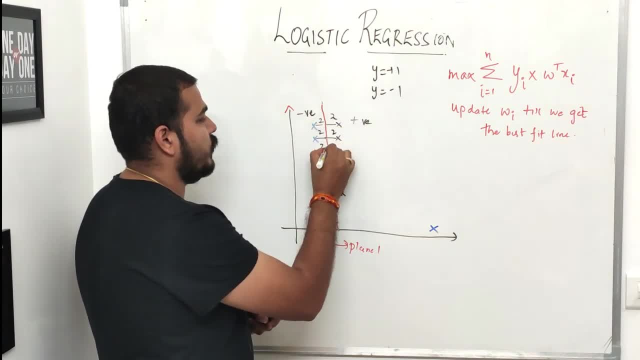 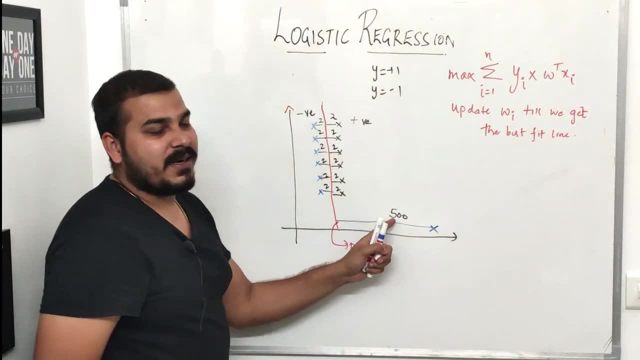 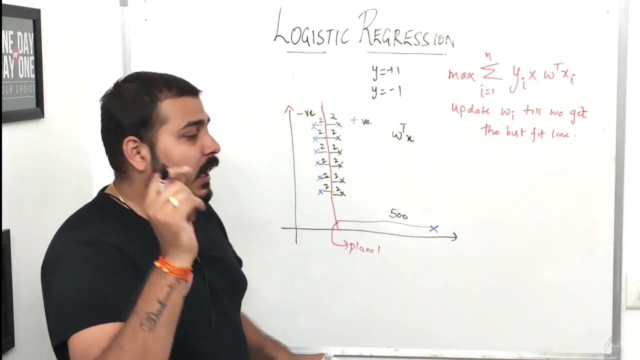 i'm just considering the same distance. okay, so this distance is two, two, two, two, two and consider that this particular distance is somewhere around 500. okay, so this particular distance distance basically means what wt of x? okay, that particular value is 500 over here. now understand that. 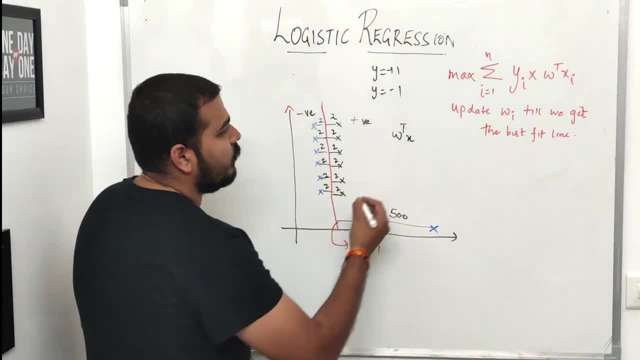 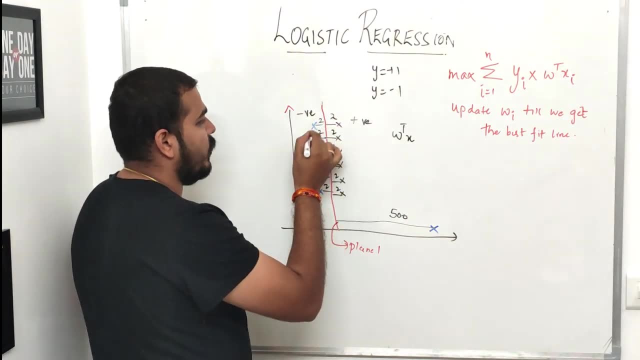 let, let us go and do the summation now, when we want to do the submission. what will happen? let us go and add this, all things right now, when we are doing the summation. this is my two, right, this is basically my two. and remember, guys, this is negative two. sorry, this is negative two because 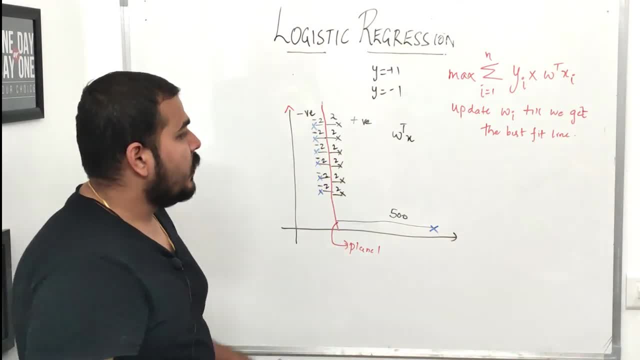 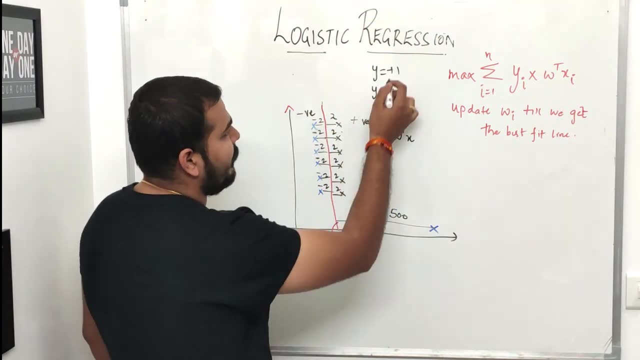 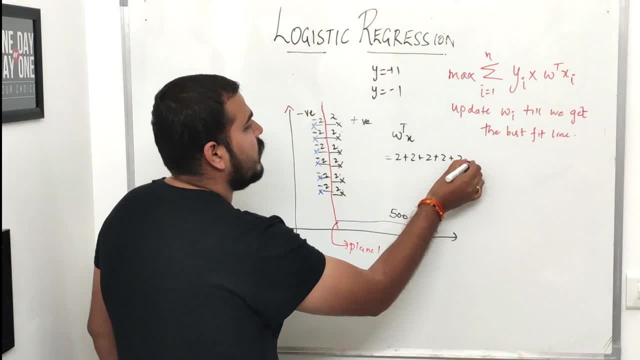 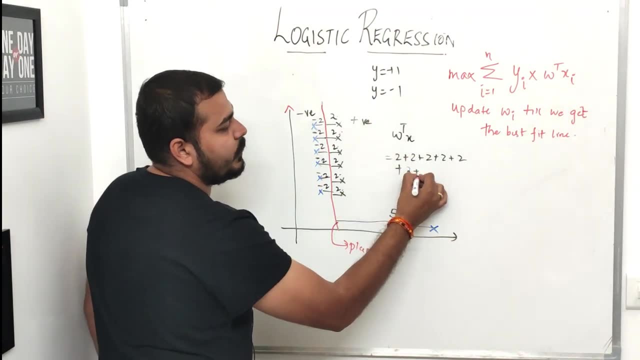 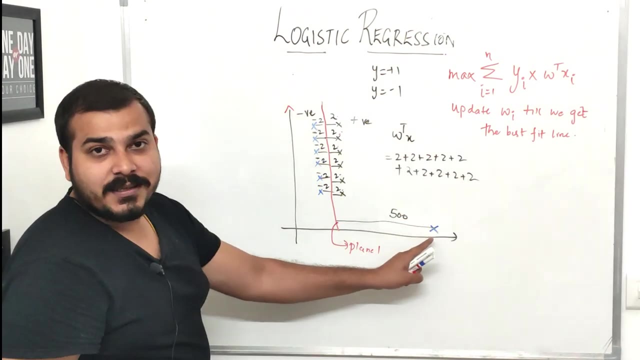 plus two, plus two, right, so they are some fine twos. now, when i'm adding this, this minus two will get multiplied by y, right? so it is nothing but minus one. so this will also become plus two, right. so total value over here you can see that it is 20, but we need to still add this, this blue. 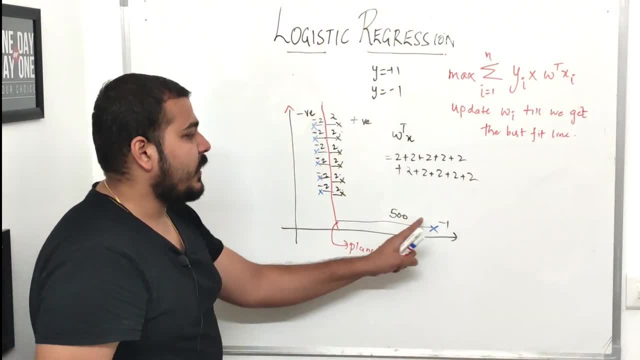 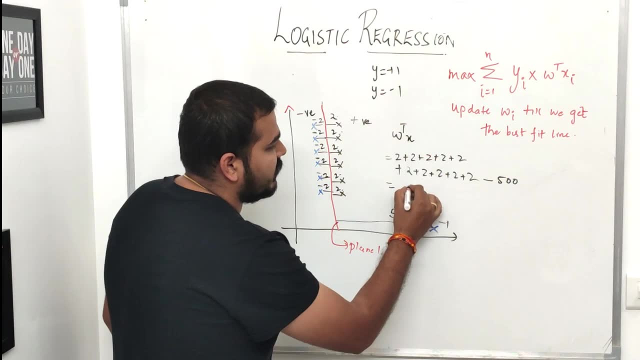 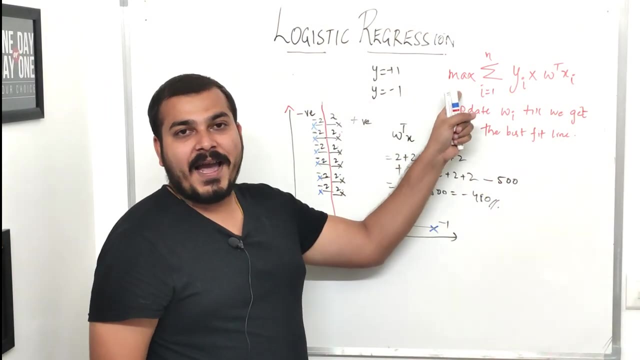 point is basically negative one, right? so negative one into 500 is nothing but minus 500. right now, when i am doing the summation of all these things, this is 20 minus 500, which is actually giving me minus 480. now, as i told you that we need to find out the max, 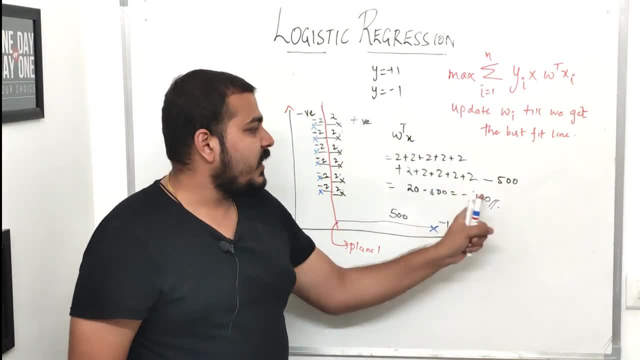 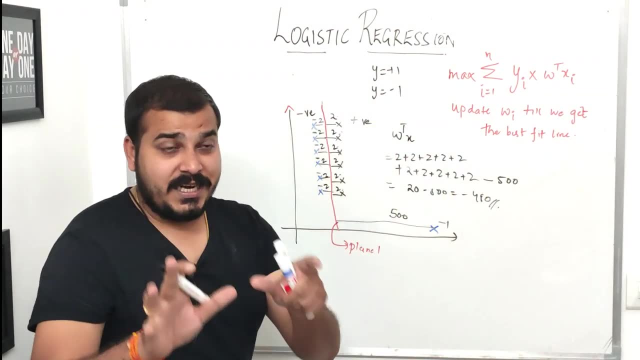 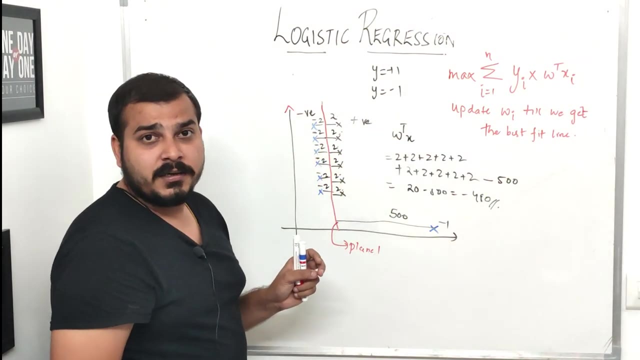 of y of i and wt of x of i, but here we are getting a negative value. so what will happen in this is that we will just skip this line. but logically, if we see that this particular line is the best fit line, right, it is easily. we are able to classify all these particular points, right, that is what we. 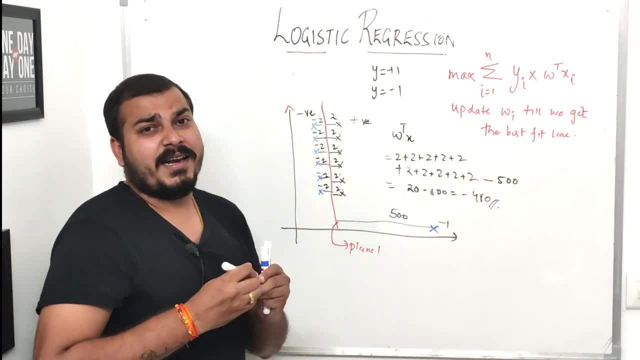 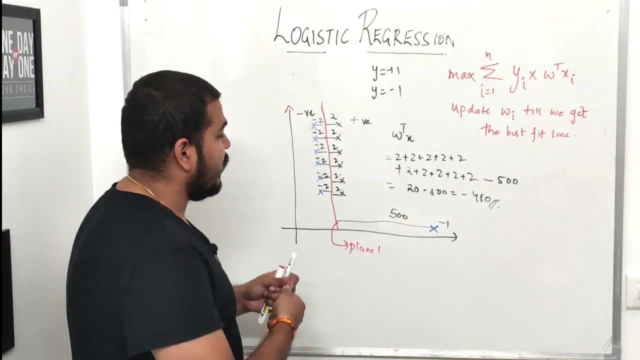 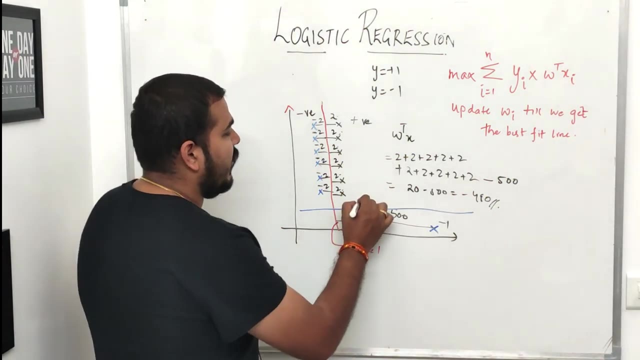 actually see right now. consider us another second line. okay, this is what is happening, guys, because of the impact of outliers, this is what it happens now. consider that i'm creating another, uh, best fit line which looks something like this. or my another plane is something like this. okay, so this plane basically indicates that above this are all. 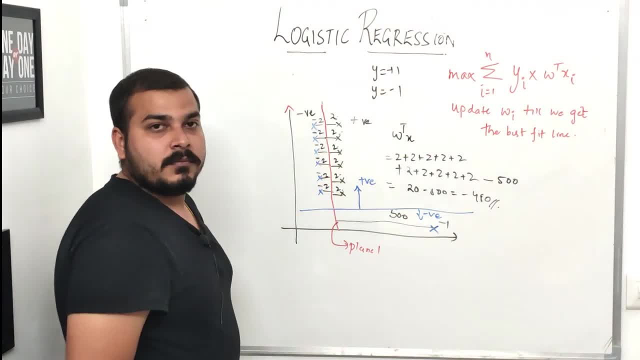 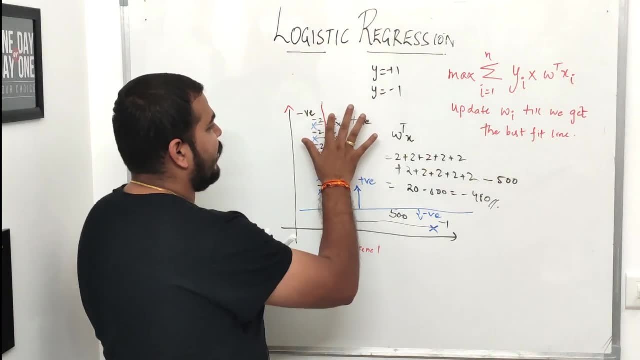 positive points below this are negative points. right now, in this particular case, what will happen is that understand one thing over here. okay, let us do this submission. okay, first of all, let me just rub all this particular value. okay, now suppose i calculate the distance between these two points. 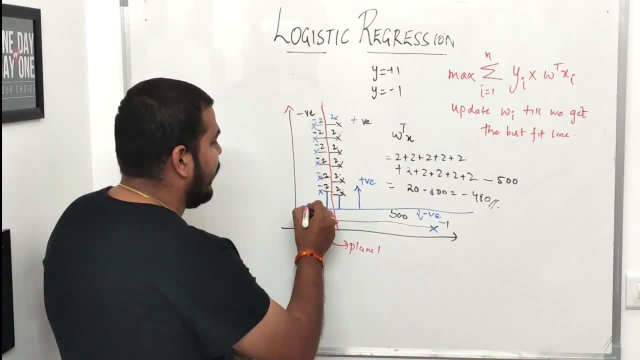 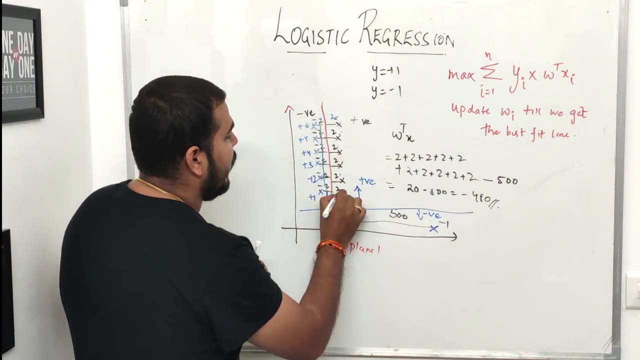 between this point and this point. okay, now suppose i calculate this is plus one, this is plus one, this is plus one plus one, two plus three plus four, plus five plus six. i'm calculating the distance like this: okay, suppose this is my distance, like this, okay. similarly, if i calculate a distance like this: 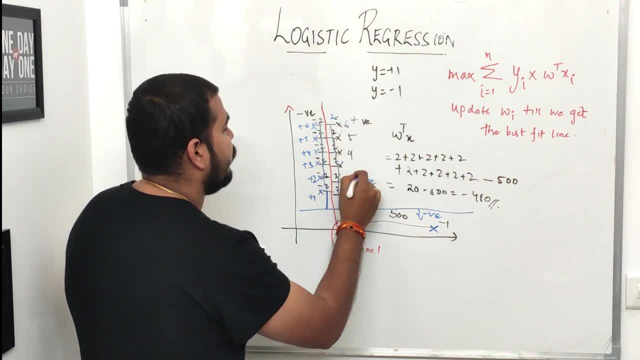 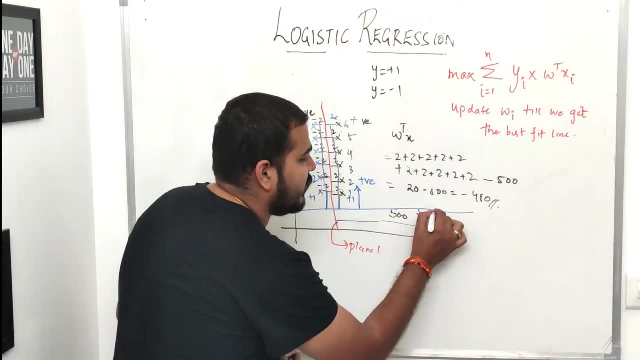 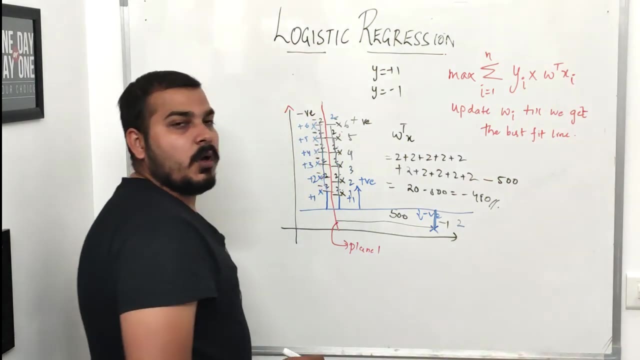 it will be also same: six, five, four, three, two, one, right now, what will happen? let me just add it up, okay, and i know this, this particular distance, this particular distance, let me consider that, uh, it is somewhere around uh, two, okay, minus two, sorry, the negative distance, okay, and these all are positive. now let me do the summation of all this. 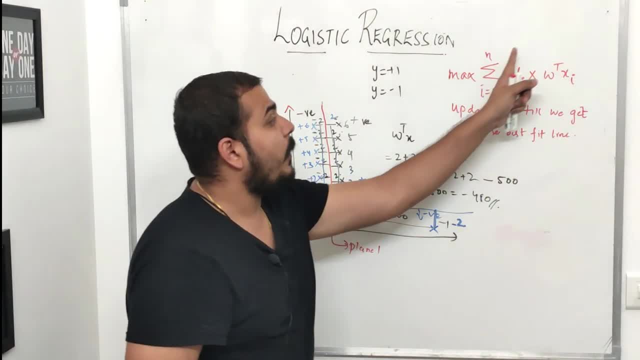 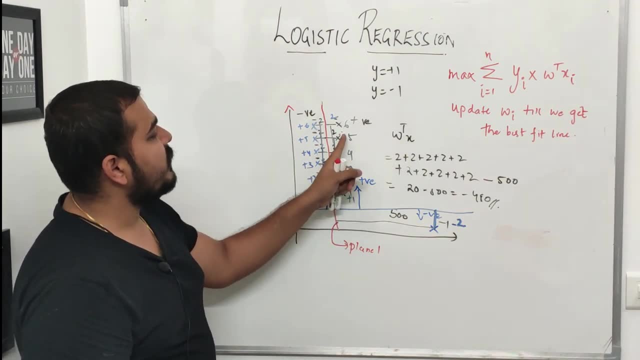 y of i, w t of i. now let us go ahead and try to apply this particular equation. okay, i have found out the distance. it is plus one plus two plus three plus four plus five plus six plus one plus two plus three plus four plus five plus six. okay, now, if i want to do the summation first of all, 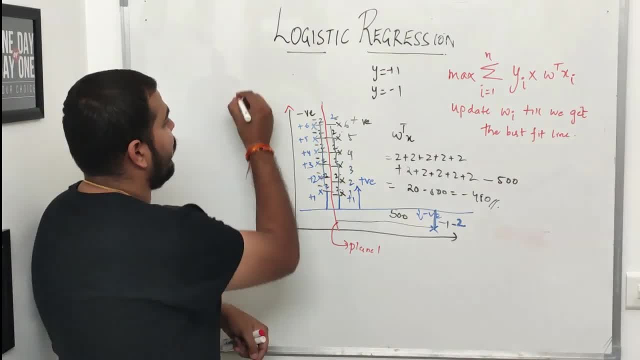 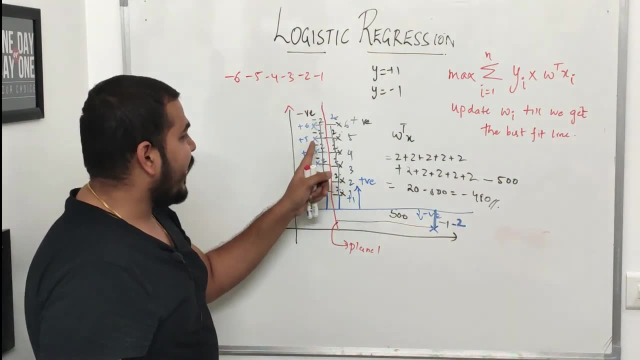 y of i multiplied by distance. i'm going to do the summation of all this y of i multiplied by distance. okay, so this will become minus six. okay, then it will become minus four, minus three, minus two, minus one, because y for negative point is minus one. remember, these blue points are basically my 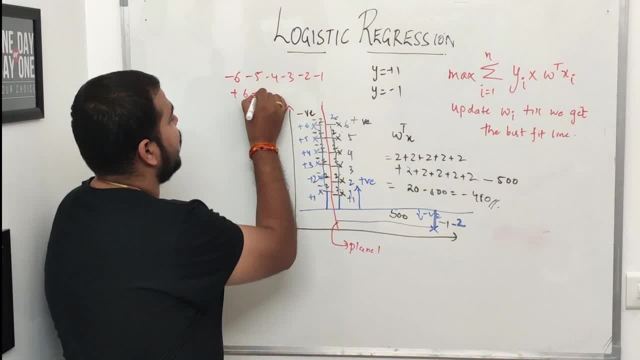 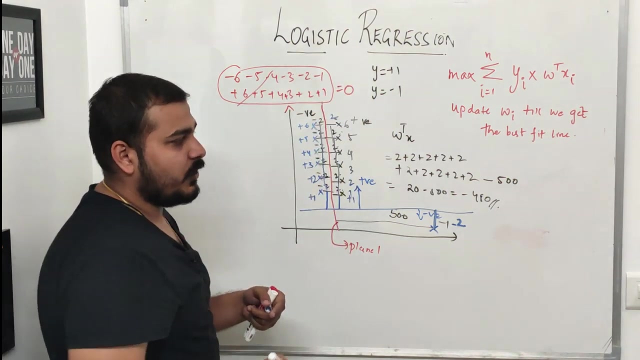 negative points. right, so minus one. after this, we'll be having six plus five plus four plus three plus two plus one, because over here y is nothing but plus one. now, when we do this, when we do this, right, it will become zero. right, we? we are basically calculating: this whole value will become zero. 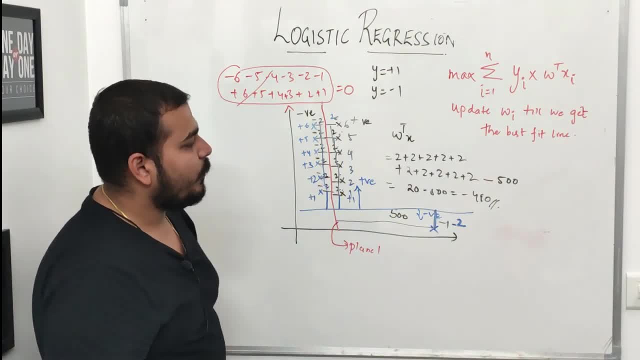 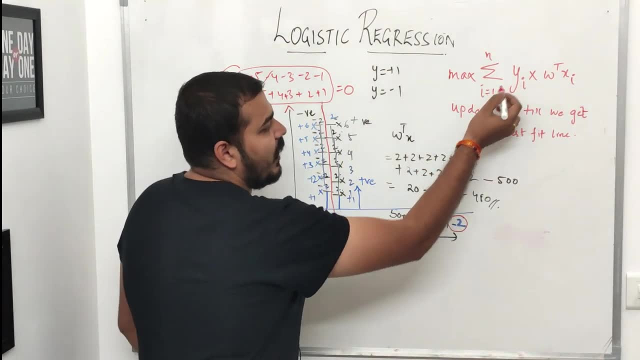 but still, there is one more point over here right now, in this particular one more point. what is happening? we are actually calculating this particular value with minus one right. minus one is my negative value. so y of i multiplied by two minus two is nothing but two. so if we 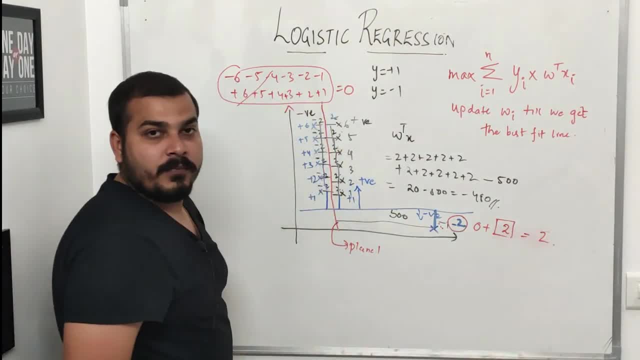 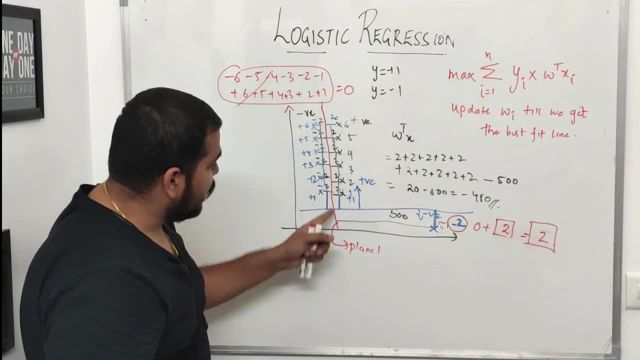 add zero plus two. this will basically be giving zero. now you can understand, guys, when we are doing this max of this. i'm getting a positive value over here, but with respect to this best fit line, i got a negative value of 480. so what will happen this? 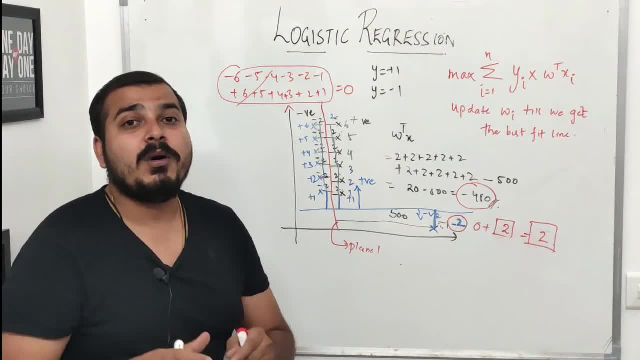 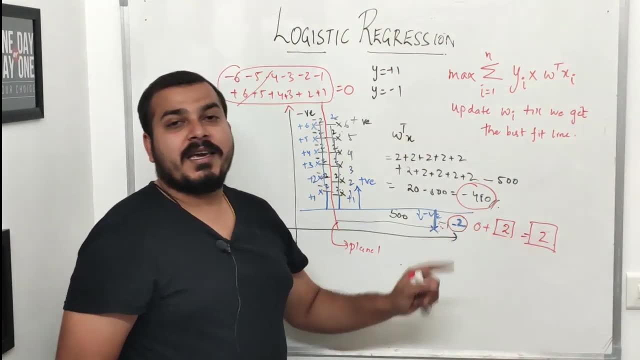 particular best fit line will get selected, and this is the impact of an outlier. this is all because of this particular outlier. what is happening for this particular case? i have got plus two, but for this particular case, i have got minus 480 right. so how do we prevent this? 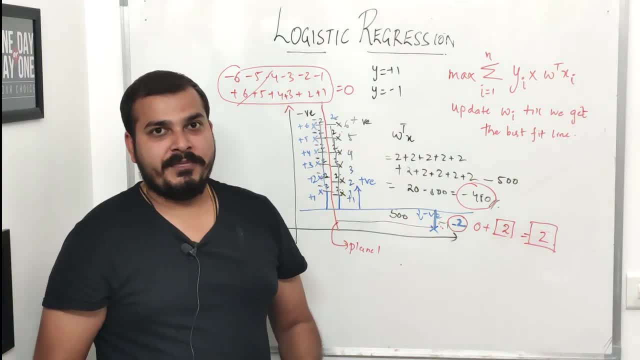 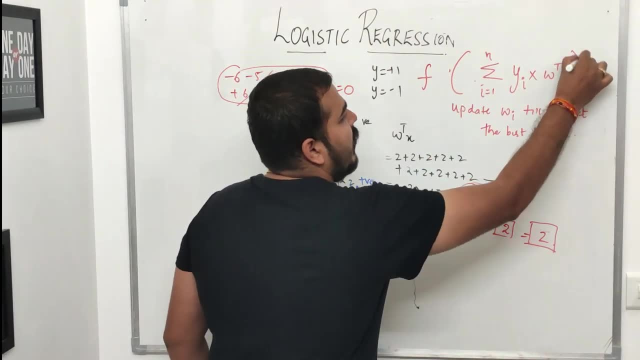 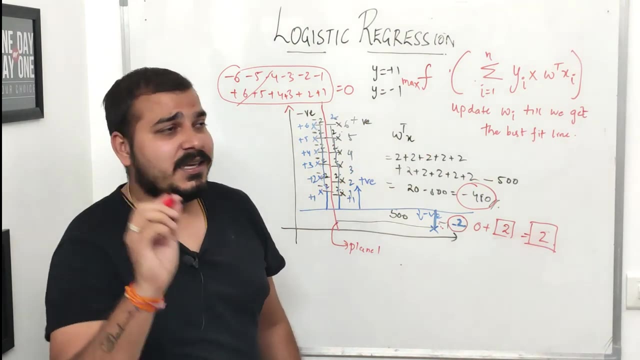 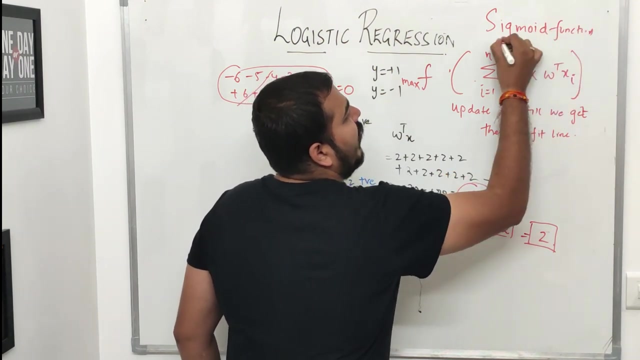 how do we prevent this? that is the most important thing for this. we just modify this equation by applying a f function around this and we actually calculate the max. now, what is this f function? this f function is nothing but sigmoid function. sigmoid function. once we do the calculation again, i'm going to remove all this particular stuff. 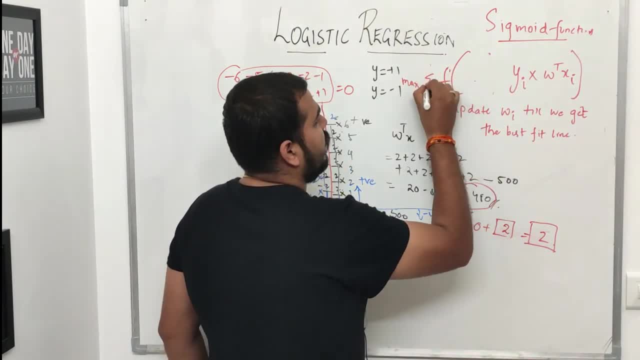 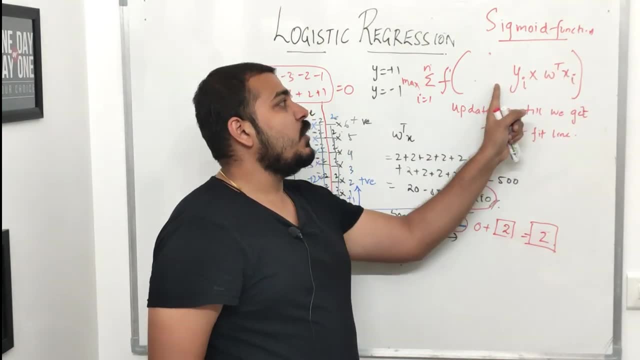 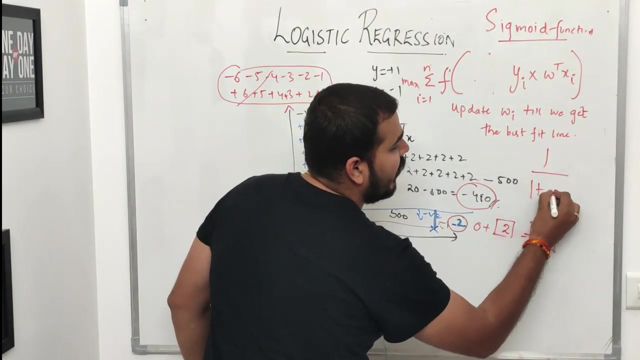 and just let me write it as like this: i is equal to one to n, right. when i am multiplying this, then this value is actually passed to the sigmoid function. now, what is the sigmoid function? remember? sigmoid function is basically given by one divided by one, plus e to the power of minus x, right, and this x. let me just 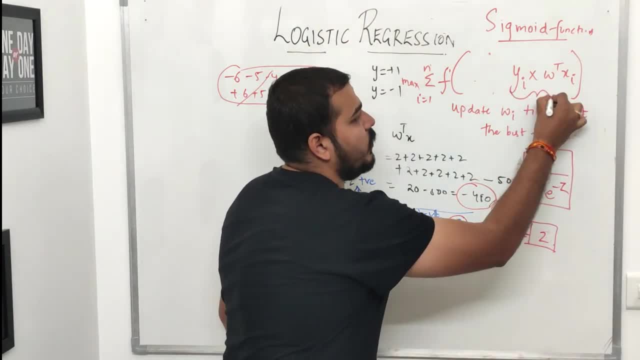 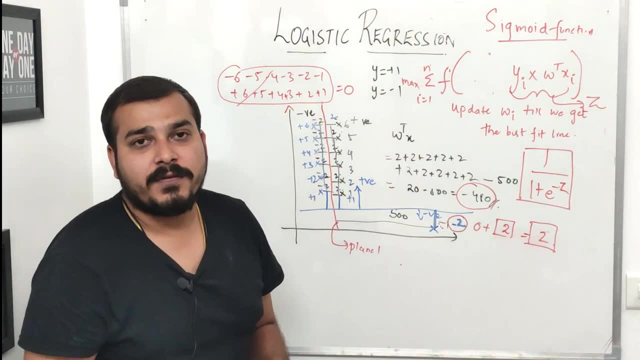 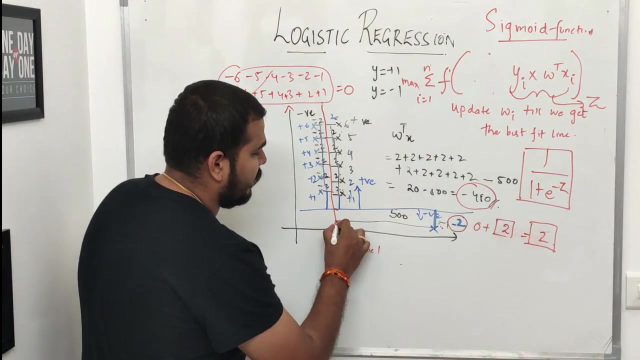 consider: this is my z and this particular value is represented as z, and we will try to place this over here. now. what is the speciality of sigmoid function? remember, guys, this distance that you see right over here, from here to this particular point, right, sorry, from here to this particular. 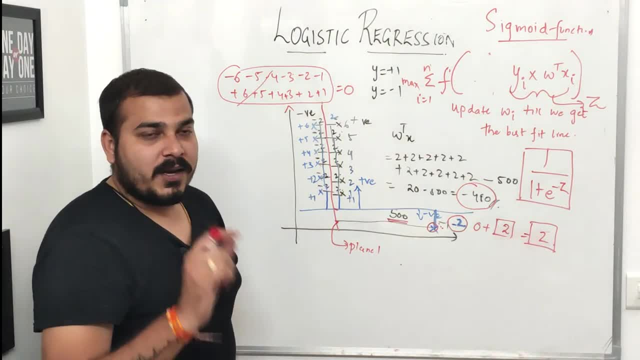 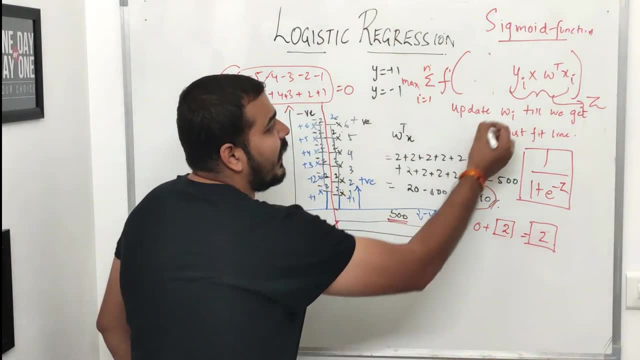 point. we saw that it is 500 right now because of this particular outlier. we are going to be able to calculate this outlier. there was a bigger impact wherein we skipped our best fit line. now, when we are actually multiplying w of i, wt of x of i, in this particular case we were multiplying 500. 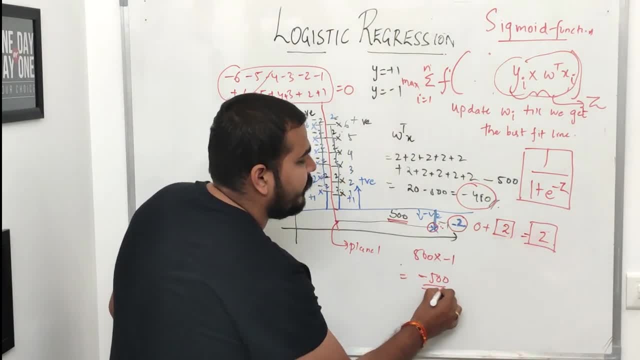 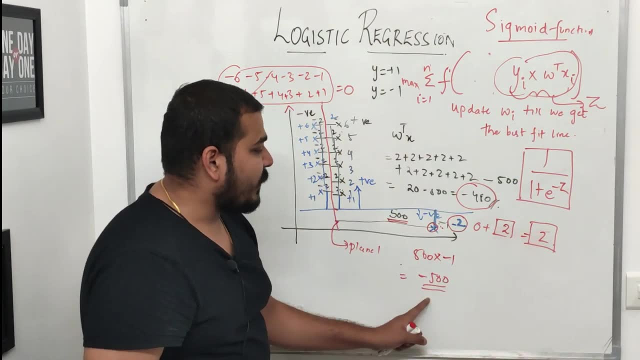 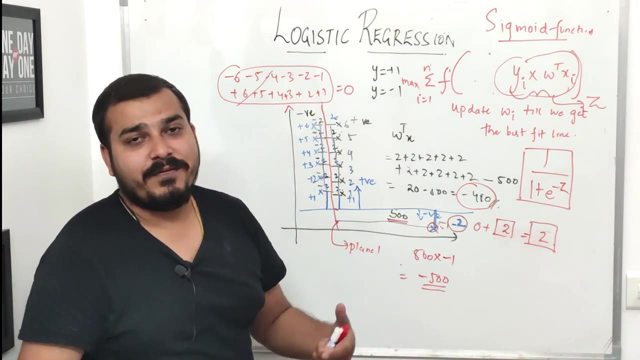 multiplied by minus 1, which is nothing but 5 minus 500. sorry, in this particular case it was positive. okay, this was negative, fine, so minus 500. now, when we got this minus 500, it is a very, very big number and when we are trying to do the summation, it basically gave us a very, very high negative. 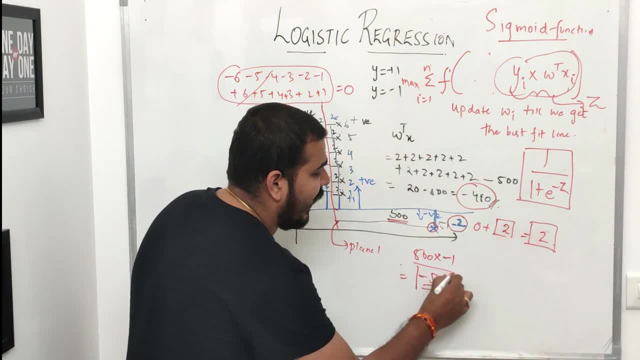 value. so we are going to be able to calculate this outlier, and we are going to be able to calculate this outlier right now. because of this, what we do is that, after calculating this value, we pass it to a sigmoid function. now, this sigmoid function will make sure that 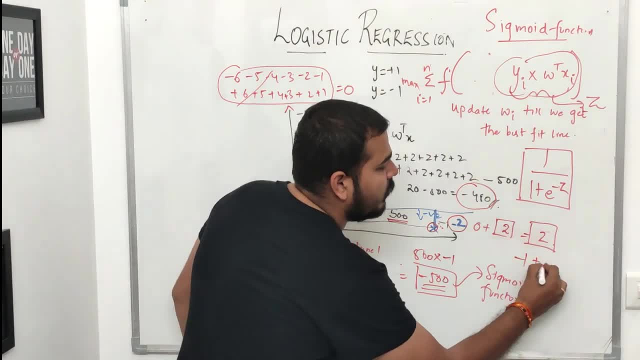 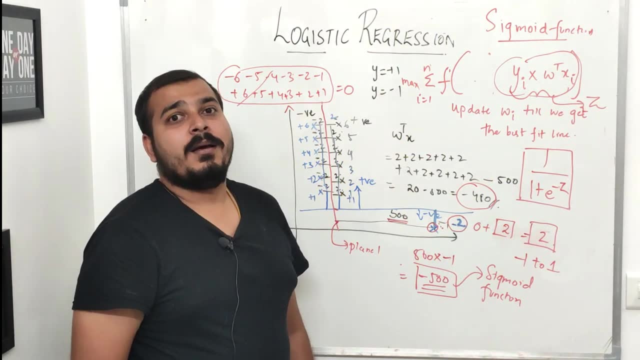 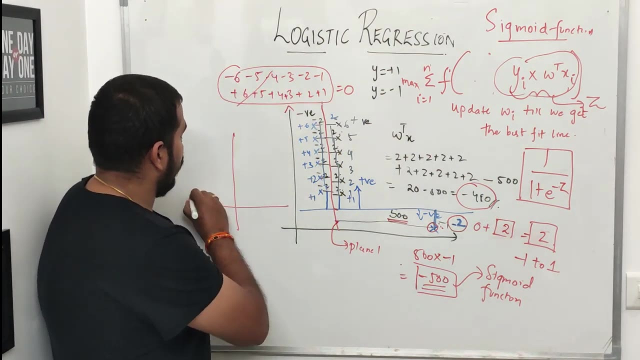 the value is transformed between minus 1 to plus 1. okay, this whole value is actually transformed between minus 1 to plus 1, and usually what we do is that for a sigmoid function, we give a very, very good equation which looks something like this: okay, so that basically means: this is my 0.5, this is my 0, this is my positive values, this is my. 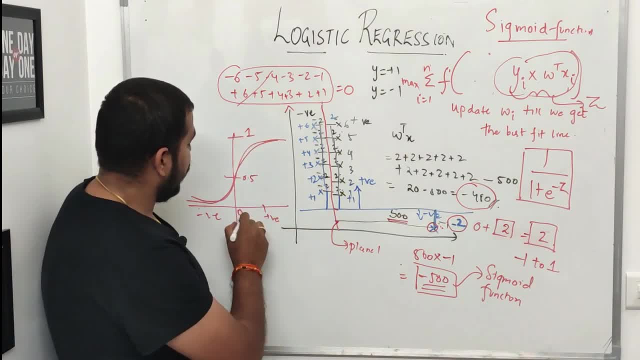 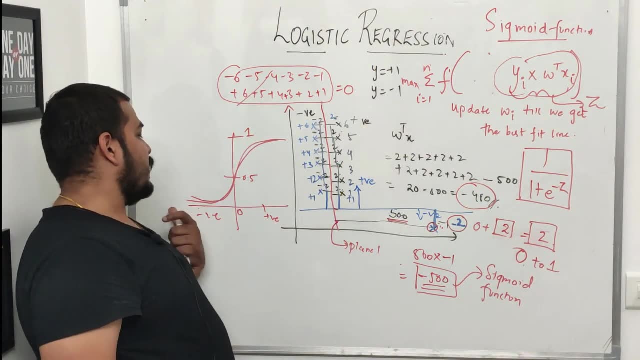 negative values, so it will be between 0 and 1. sorry, it should not be between minus 1 to 0, plus 1 between 0 to 1. i can also say minus 1 in this particular value, but it will always be between 0. 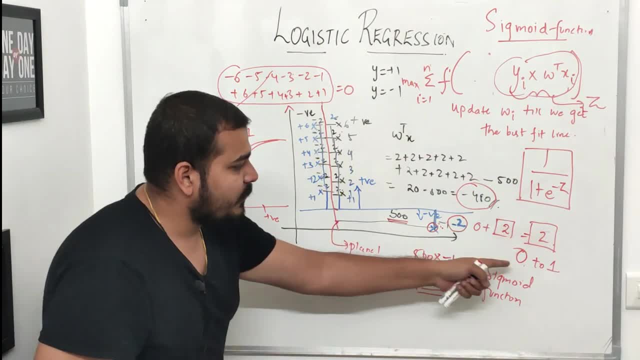 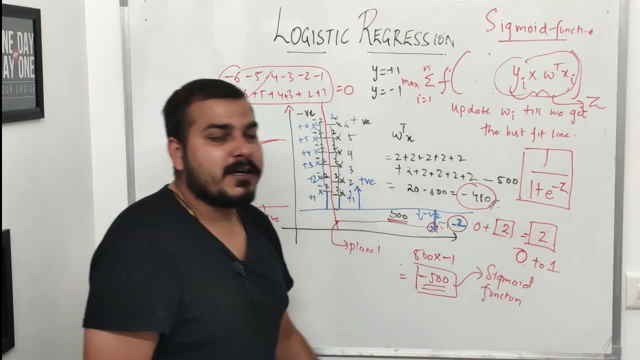 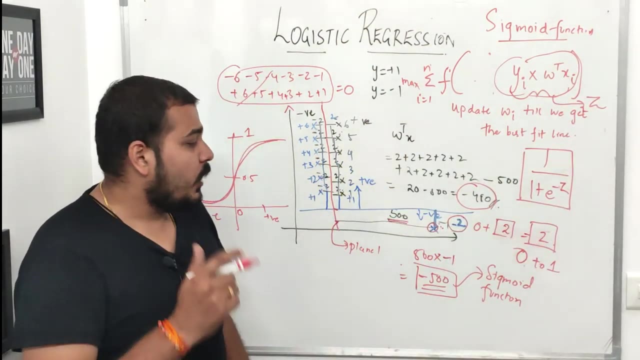 to plus 1. okay, and always remember, guys, if i want to consider minus 1 to plus 1, there is another function which we will be discussing that in the future classes. but just understand, a sigmoid function will actually transform all your summation between 0 to 1, not summation, this multiplication between 0 to 1. now, when it is doing that, 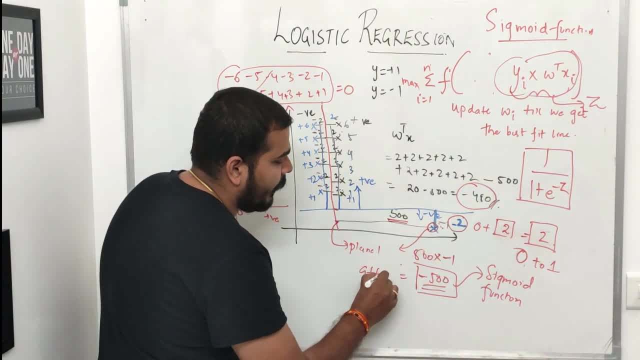 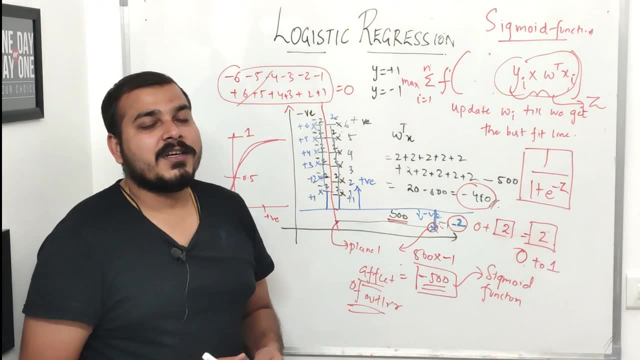 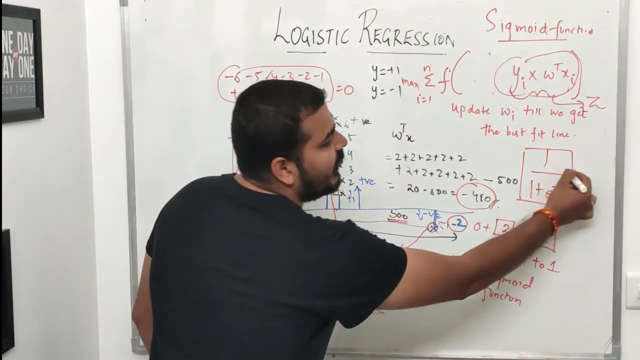 it is removing the effect of outlier. it is the removing the effect of outlier and that is where this sigmoid function is actually used. remember this particular stuff, guys. this is the diagram we usually. we give the equation- i have defined it over here- 1 plus e to. 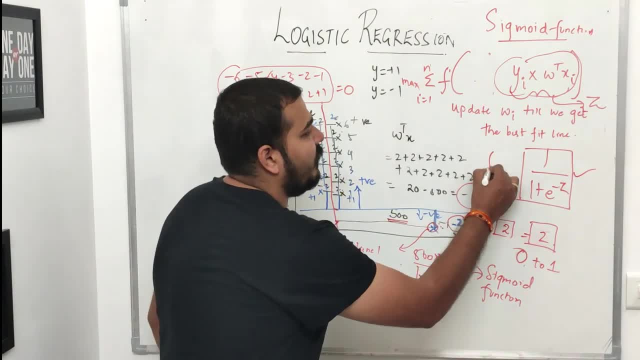 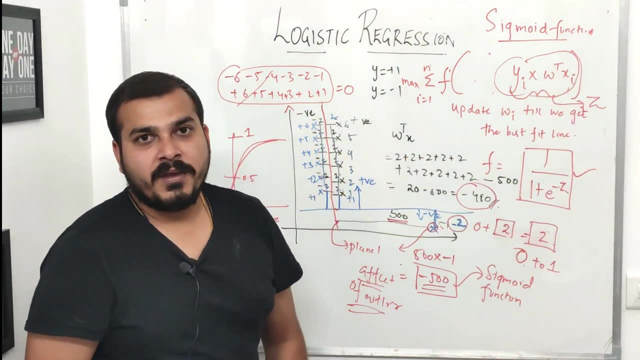 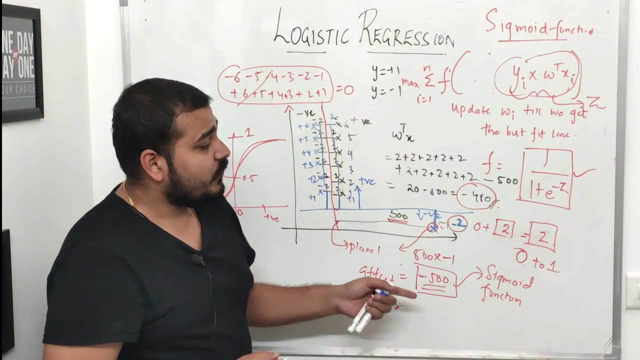 the power of minus z. this f is nothing but this particular value, okay, and this z is actually replaced with the multiplication of y of i and wt of x of i. now, this is why we exactly use this sigmoid function, and this is actually transforming your value between 0 to 1. how much high value may be having? 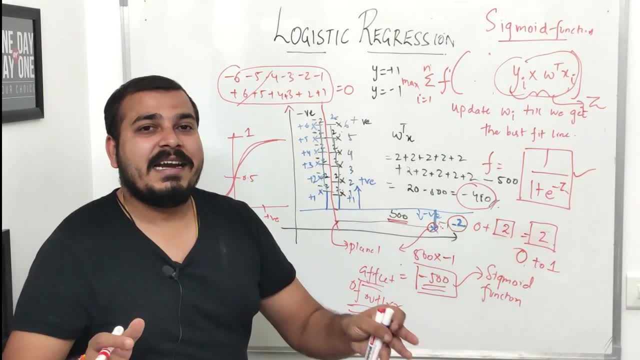 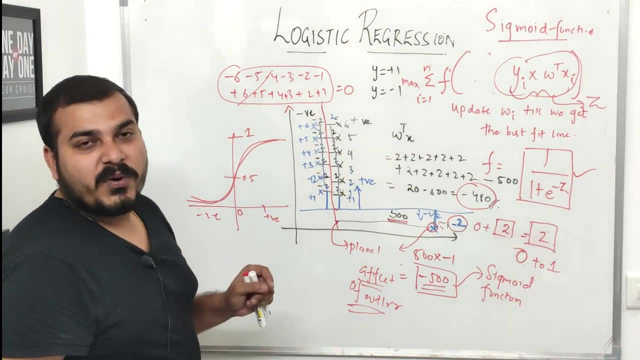 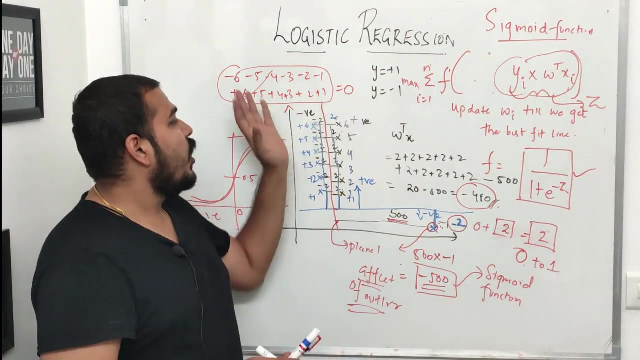 let it be any number of outliers you have. it will directly transform those values into a very, very smaller value that will range between 0 to plus 1. pretty much simple, pretty much amazing guys. so this is how you should actually understand about the logistic regression. this is how you actually go through it. you know the main funda of actually. 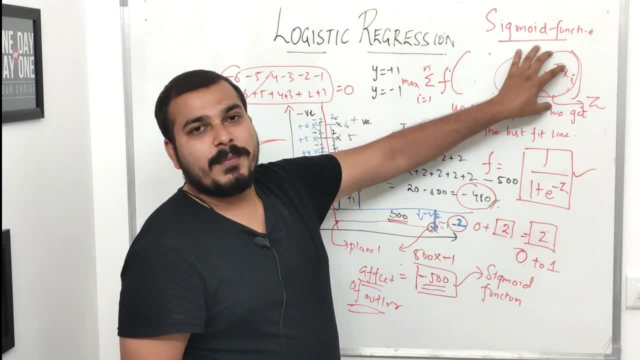 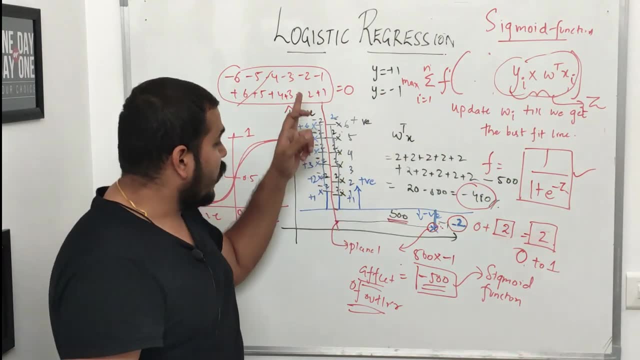 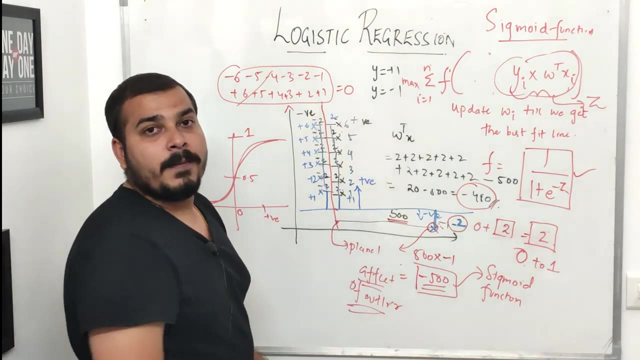 finding the best fit line is basically doing this multiplication and then applying this particular activation function, updating this w value unless and until you don't get a best fit line that can classify this point. and always remember, guys, this max is pretty much important. the summation of all this particular stuff, all these particular points, along with this distance, 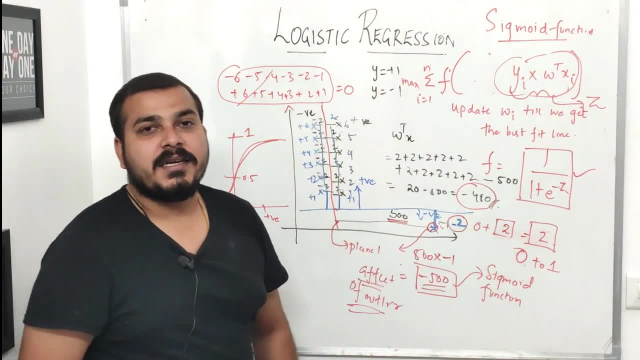 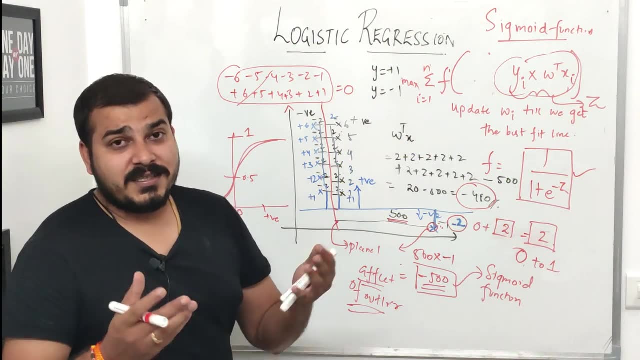 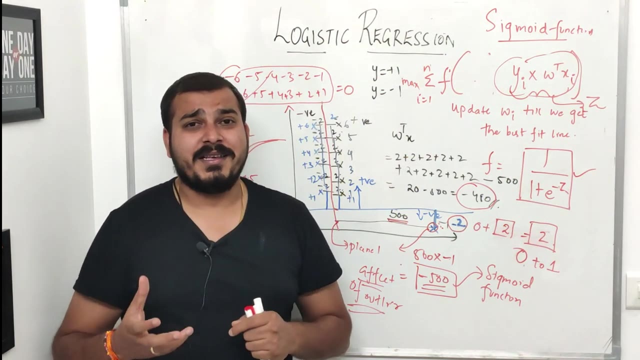 should be maximum, then only that particular line will be considered as a best fit line, which will actually classify the points separately easily. okay, so yes, uh, this was all about this particular video. again, in the part three i'll be also coming some more explanation about logistic regression. there are some important things. uh, what is regularization and all that i'll be explaining. 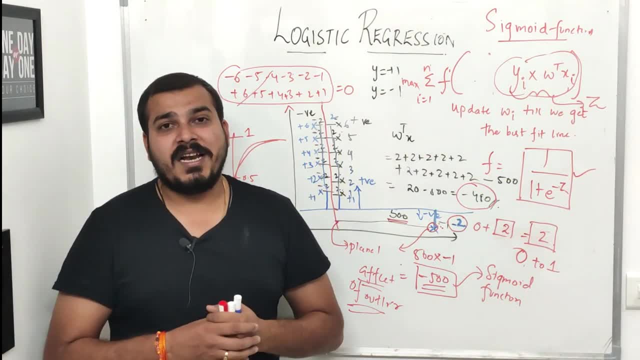 in the part three. i hope you like this particular video. please do subscribe the channel if you have a not already subscribed. i'll see you all in the next video. have a great day. thank you, one and all bye.